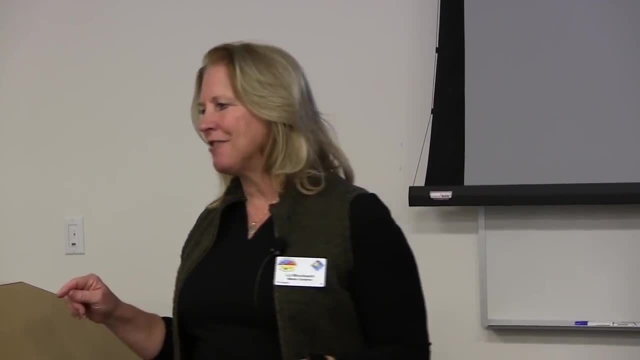 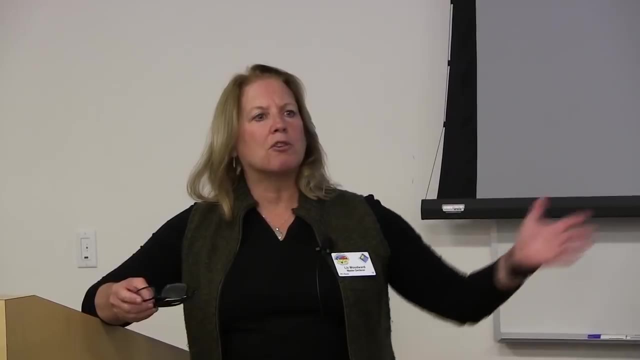 rarely actually get a hotline call on any specific thing in that chapter, so rest assured of that. So we're going to try to drill that down to what is important for you as a master gardener in understanding what some of these principles of horticulture are. that will fall. 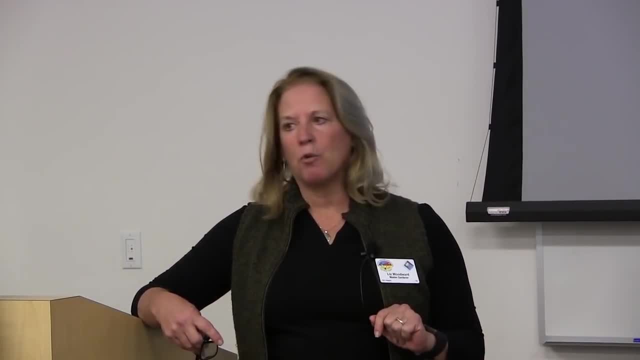 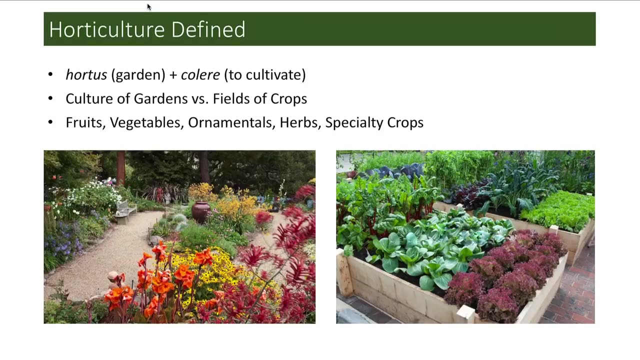 into play as you go further in and that type of thing with the course. So that's what we're going to do, where we're heading. Again, we're going to be talking about this is the introduction of horticulture, and horticulture is a big, long word, basically deriving from the Latin. 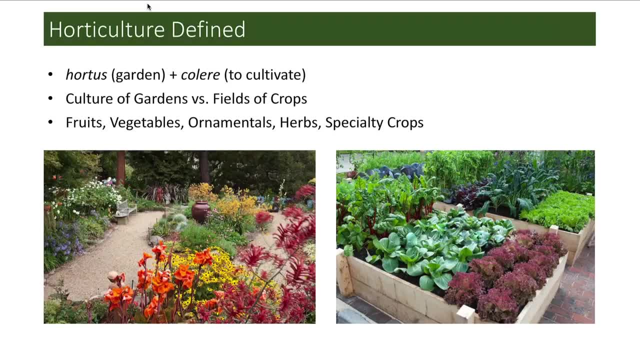 words hortus and colere, which hortus means garden and colere means to cultivate. And when you see somebody studying horticulture, it's horticulture versus agronomy, which is a study of like fields of crops which require a lot less intensive management. Horticulture- 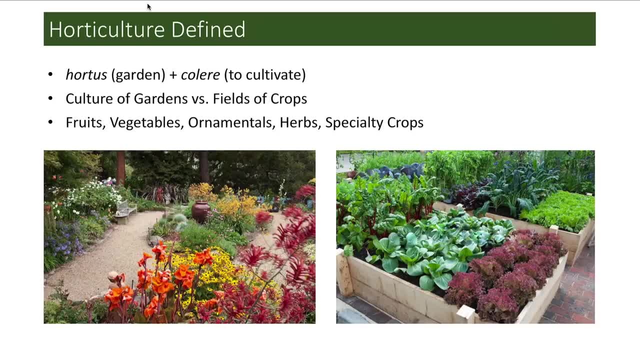 is a little bit more difficult. You're usually dealing with higher valuable type of crops, things that are more perishable. They're the type of things that we will be dealing with mainly as master gardeners. There are things like fruit gardens, vegetable gardens. 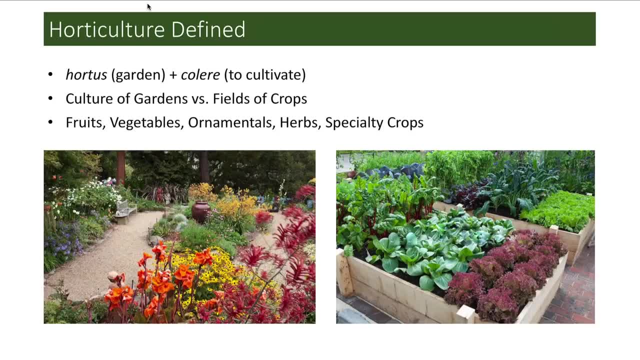 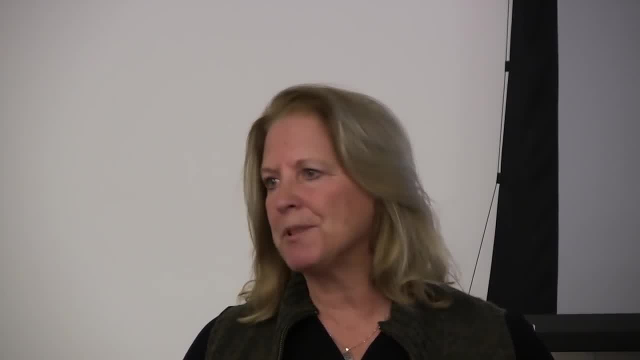 your ornamental crops, I say as a general, like your landscape plants, your herbs and your specialty crops. And again, when I say crops, I mean type of plants, Like specialty crops could mean native plants, Mediterranean area plants, as we get into more drought-tolerant. 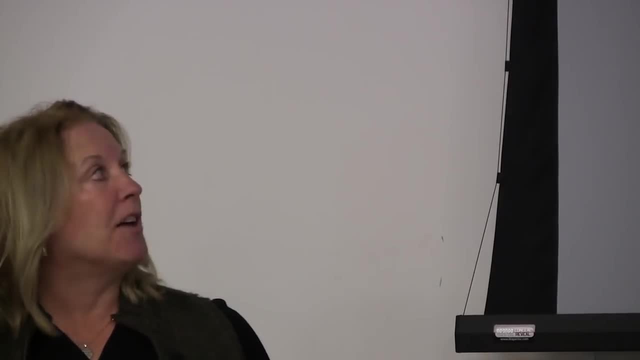 plants. So we're going to be looking at those things, And the other thing that we're going to be looking at is we're going to be looking at the understanding of horticulture. You have to understand some of those underlying principles. 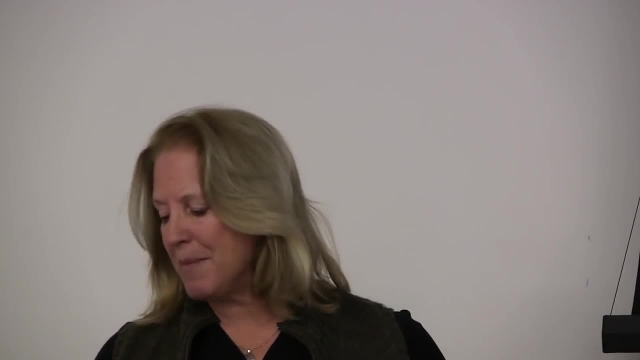 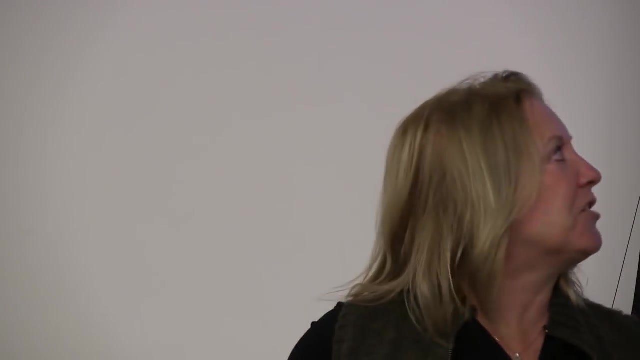 so that because it is part a science and part an art to managing these type of things, So in looking there's a lot of people that have contributed to this field. But I chose these two because I think they kind of give us the most run for our money in terms of. 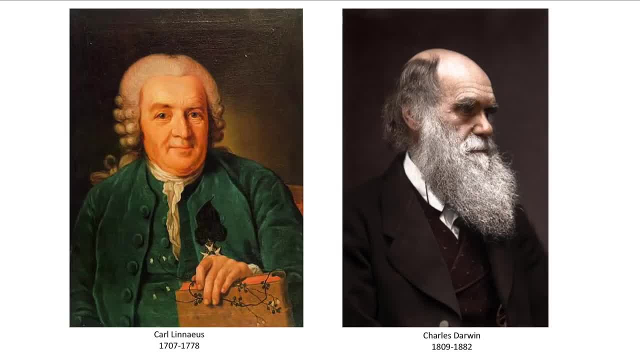 what we're looking at. Carl Linnaeus Moe is going to talk a lot about his system that he developed, But he's the guy we have responsible for all of this land development And he's the guy we have responsible for all of this Latin jargon that we use in horticulture. He's 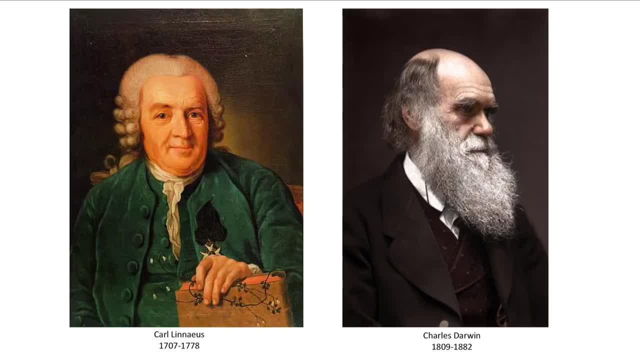 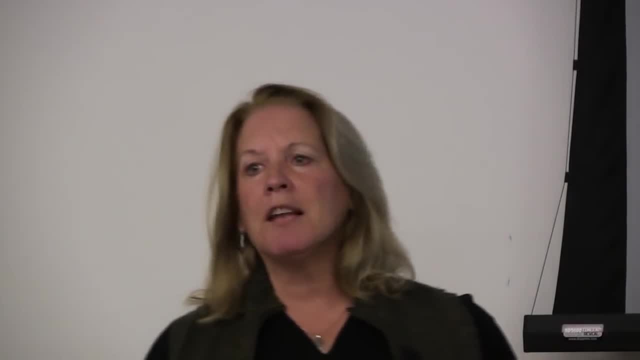 an interesting guy. He lived in the 1700s, He was a physician, He was a zoologist, He was a botanist, He was the son of a minister from Sweden And he realized in his work as a physician that you know as talking across the board with physicians from especially. 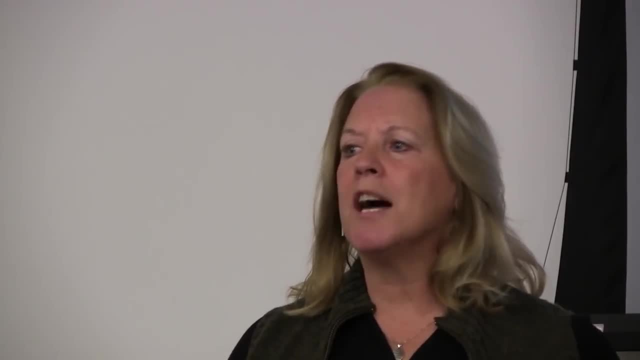 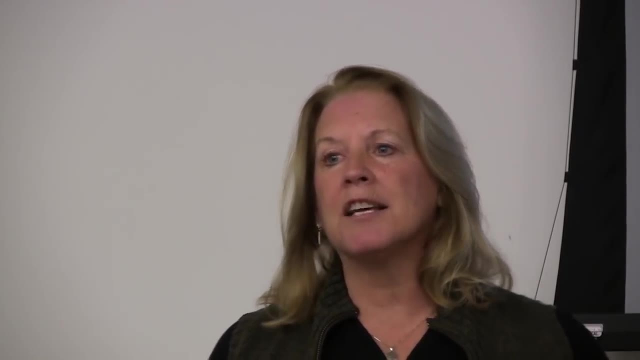 coming from Sweden, where there weren't a lot of people speaking Swedish, when doctors had to communicate, they had to communicate on a common language, So they knew that they were talking about the same thing He realized in the world of plants and animals, which is, you know, again being a botanist. 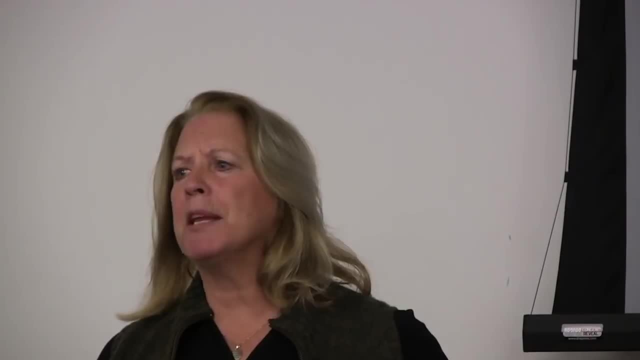 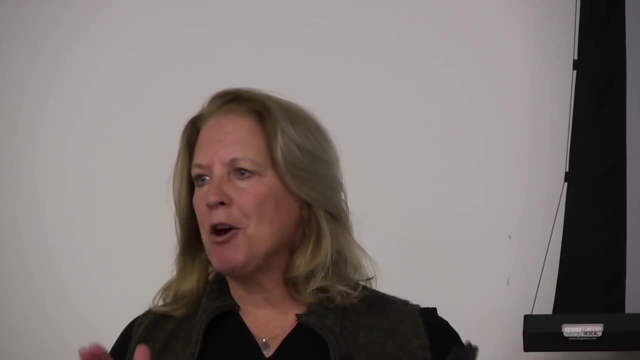 and a zoologist on top of being a physician. he realized there was probably a need to bring that kind of some kind of common naming classification there. So he developed this binomial nomenclature which Moe is going to talk about And with that he developed this way to kind of a nested 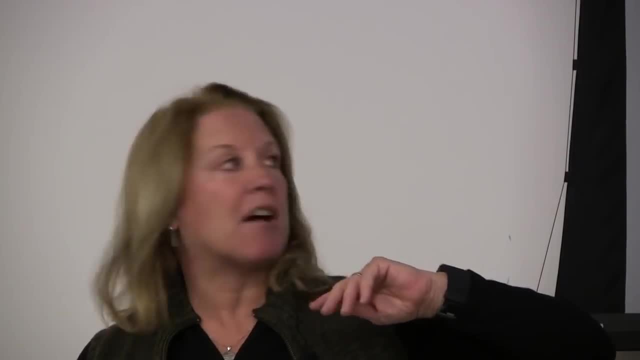 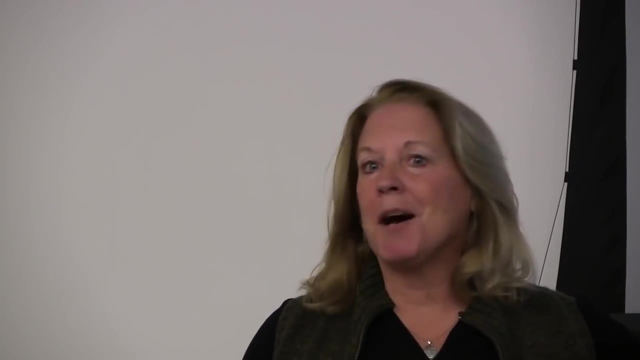 hierarchy, to kind of to differentiate down the way. So he's responsible for that. We call him the father of taxonomy. I will admit a lot of the things that in the Linnaean world that he classified have been reclassified because he didn't have the advantage that 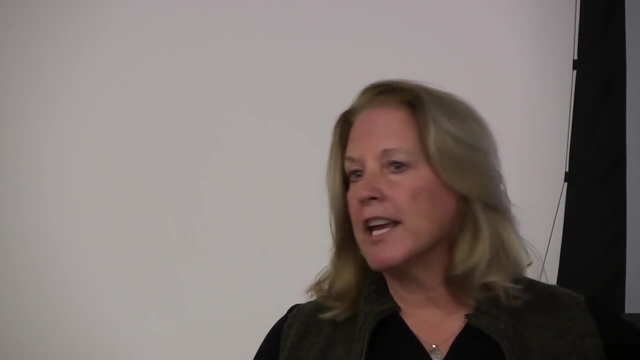 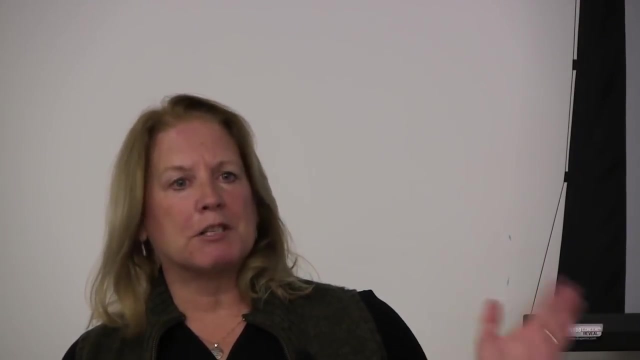 we have today even microscopic evidence or looking at DNA structures in plants. So you'll often see, sometimes people will. if you read about a plant in particular, you know specific species. you'll say: you'll see things that were Linnaeus identified it. 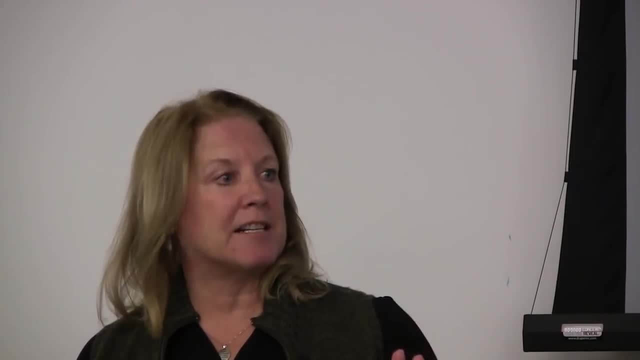 as or under the Linnaean system. they identified it as such, and it had a similar name to it, villainous one, which is a hymen, And that that was the way that they told you about nomenclature. And so he was. he continued to kind of navigate like that, And so the 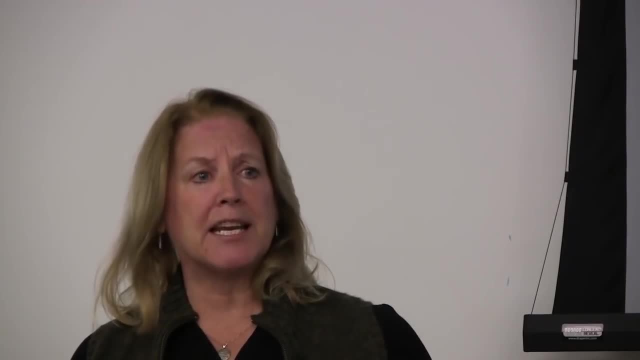 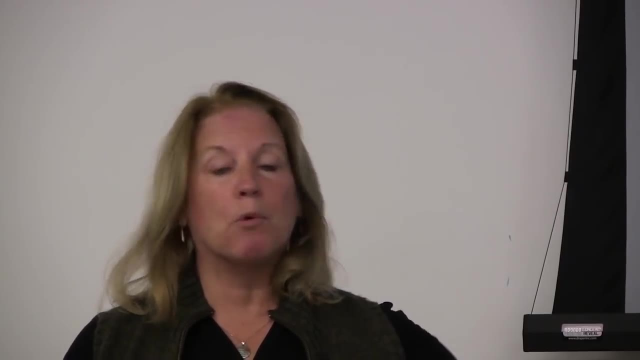 has since changed And we're especially starting to see with DNA sequencing. things are really changing a lot in the last, you know, probably in the last 15 years, 50 to 20 years more than they had in the 200 years before that. The other guy I have up here is Charles Darwin. 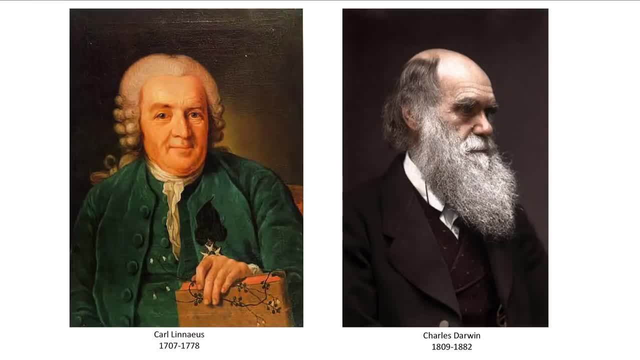 And again I look at, he was a botanist and he traveled the world and we think of him as the guy who had the theory of evolution. And he did that by basically studying plants first. When he would go off on his voyages he would see things with plants He developed. 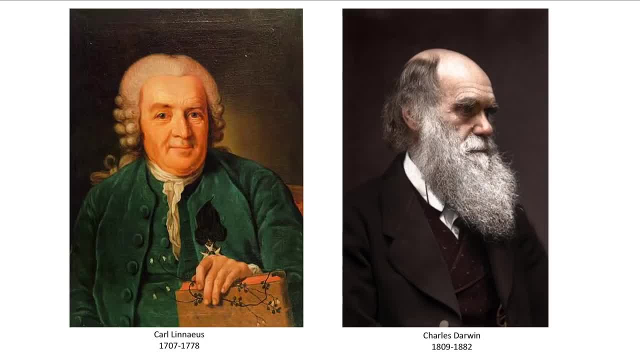 a lot of his theory about survival of the fittest and that type of thing, as he would see how plants survive under different circumstances. And so he actually, by looking at plants first, he was first before he developed that with humans. he actually developed that with plants. 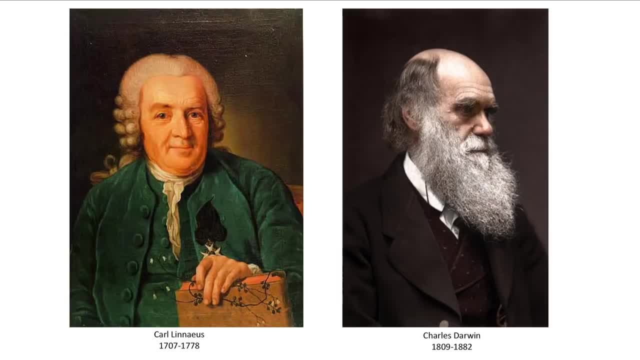 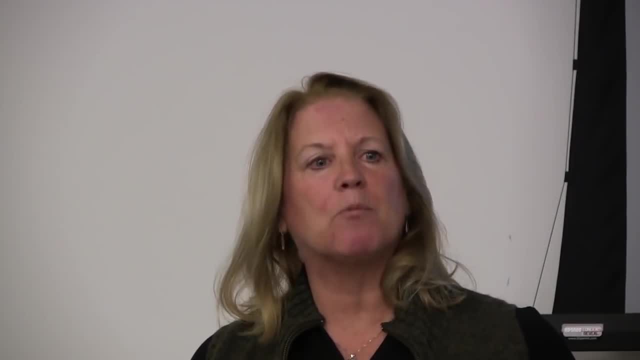 looking at the way flowers were structured and seeing how easy it was to cross-pollinate a flower and how, therefore, how plants had to survive, And he did that by looking at plants that developed systems in which they could protect themselves against cross-pollination. 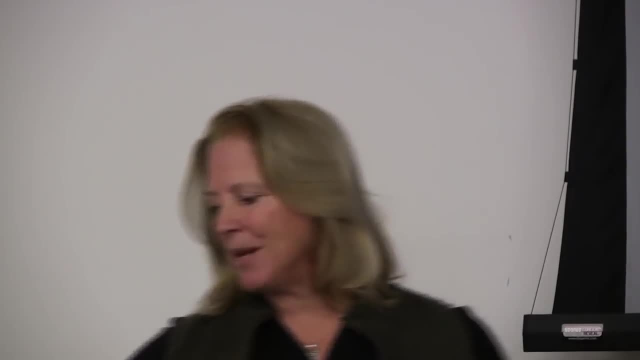 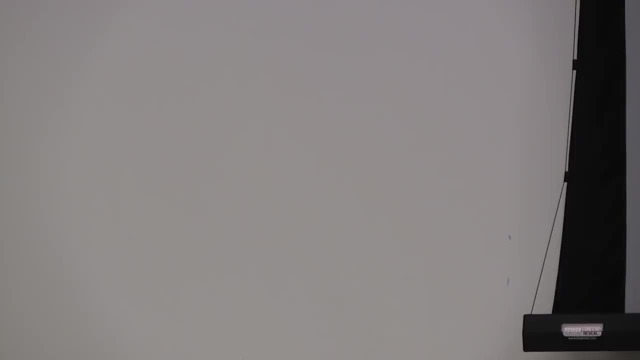 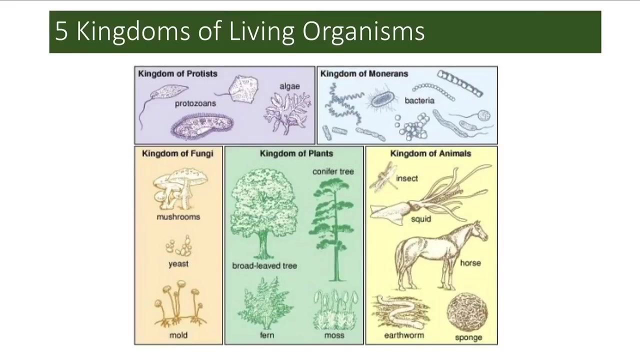 to keep themselves pure and to keep themselves viable and to keep reproducing. So Linnaeus, during Linnaeus' time, Linnaeus identified these two kingdoms, the plant kingdom and the animal kingdom, But today we have five kingdoms of living organisms. These top. 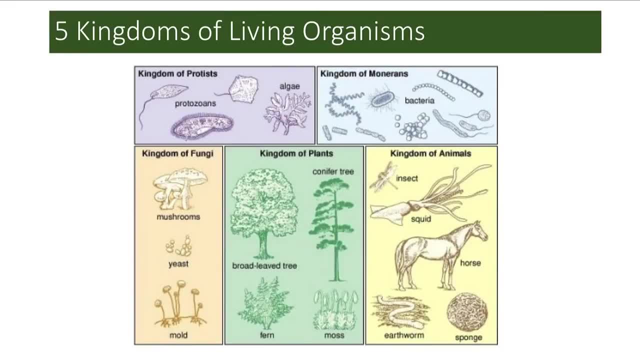 two kingdoms. they're probably the most boring. Those consist of: the top one is the lowest kingdom, the kingdom of the monarch, And those are basically. they are complex, single-celled organisms, They are your bacteria, that type of thing. The kingdom next to it, that's kind of an odd kingdom. They basically 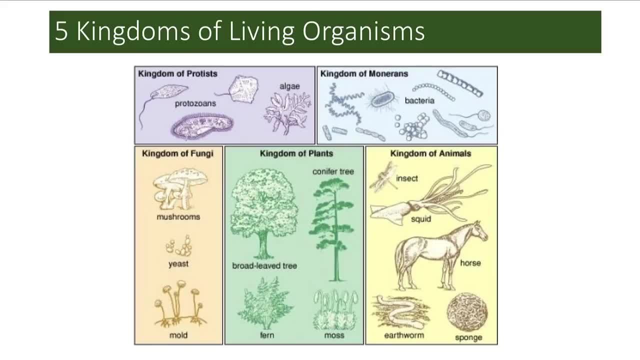 throw anything in there that's not a bacteria, that's not a plant animal or fungus is thrown into that. So that includes things like your algae, your slime, molds, all kinds of weird stuff And that will probably someday- probably scientifically- that kingdom will. 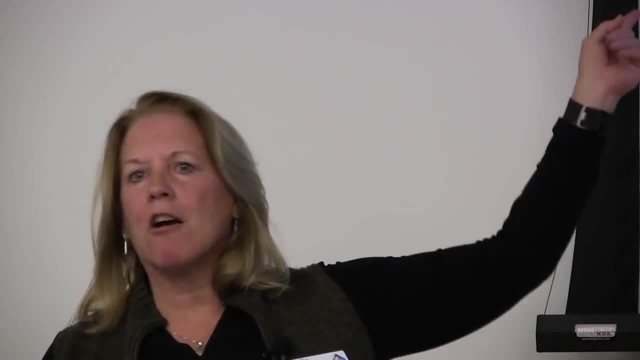 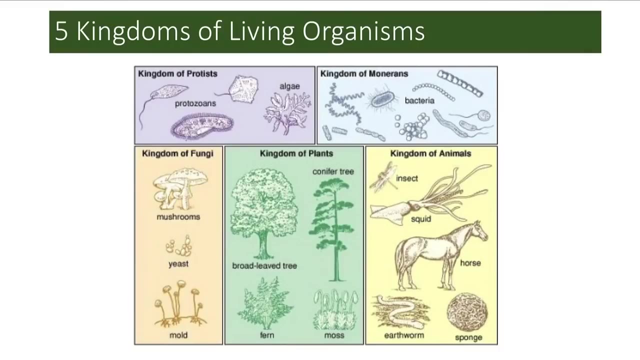 disappear And will break out as they understand those organisms. But they are also single-celled, complex organisms. We get into the smallest of these kingdoms here, the kingdom of the fungi- Fungi, as they call them often- And those are your mushrooms, your yeast, your molds, your mildews, Those 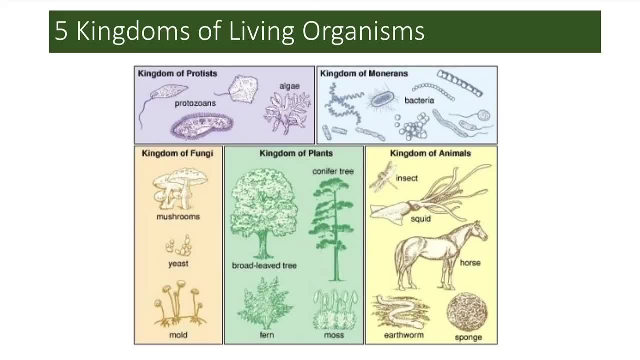 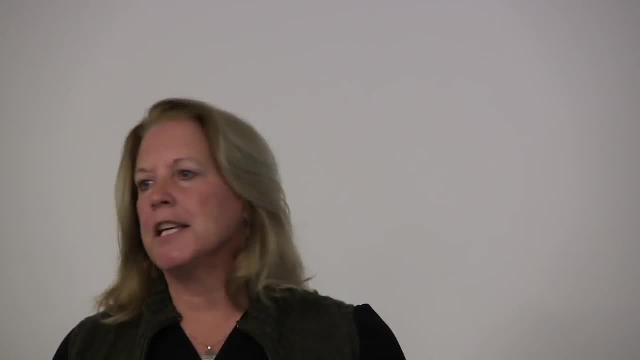 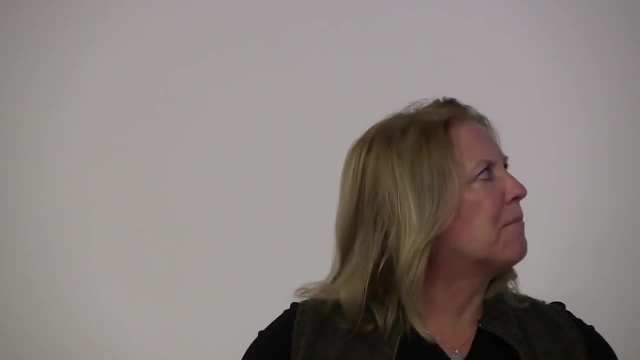 are all? they're multi-celled organisms like plants, But the thing that differentiates them from plants is they do not produce their own food, So they live off decaying matter in the air or in the soil, And that's what differentiates them. There are not that many members of them, but there 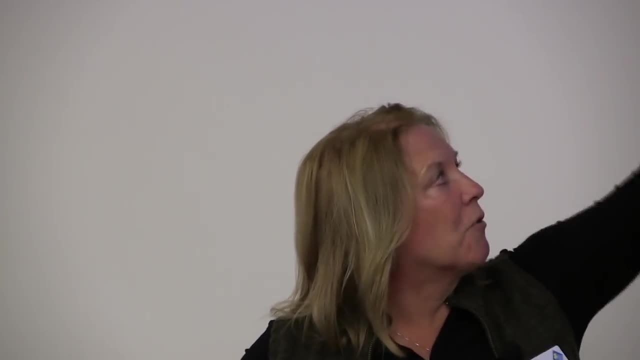 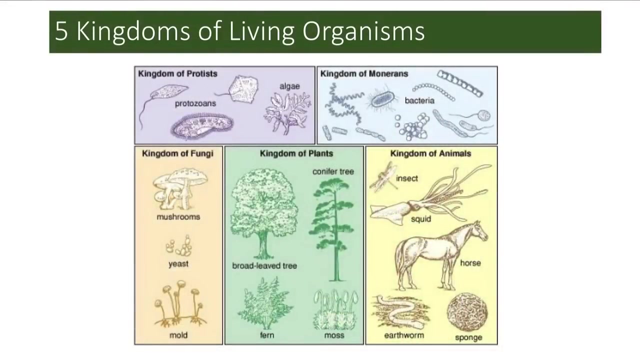 are quite less than the other two. on top The kingdom of the plants, they have probably a little over 300,000 species. They are all the flowering plants that we know and love in our garden, And they do include. the thing that makes them unique is they're multi-celled. 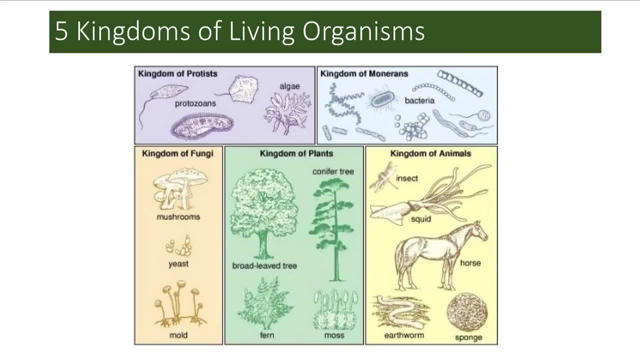 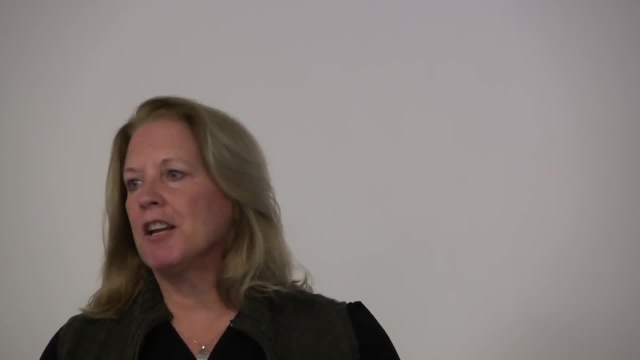 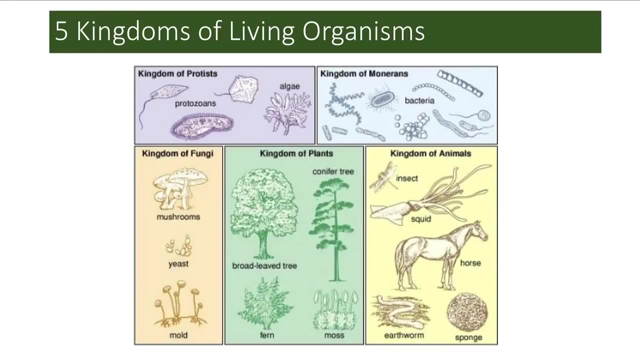 organisms They produce. of all of these kingdoms, they're the ones that produce their own food Through photosynthesis, which we'll talk about. Then. the animal kingdom is the very largest. They're the most complex. They have over a million species in there And they rely very much on the plant kingdom. They wouldn't exist. 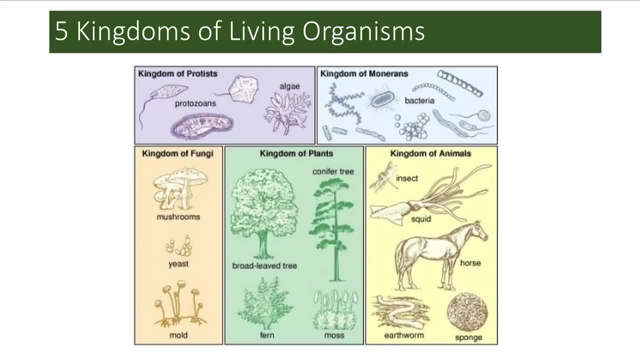 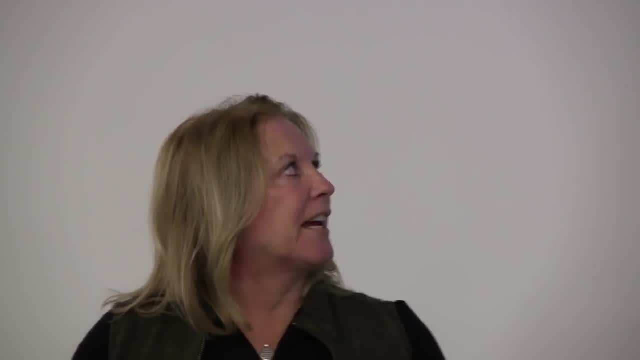 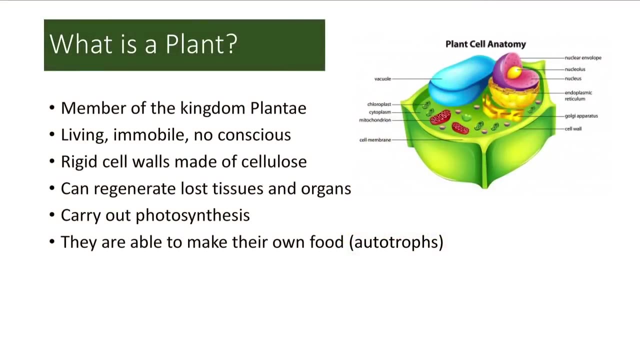 without the existence of the plant kingdom because basically anything that they eat, and wear and do is dependent upon that plant kingdom. So what is a plant? We know that they belong in the member of the plant kingdom. They're living, multi-celled beings. They're basically immobile, although we think of them moving. 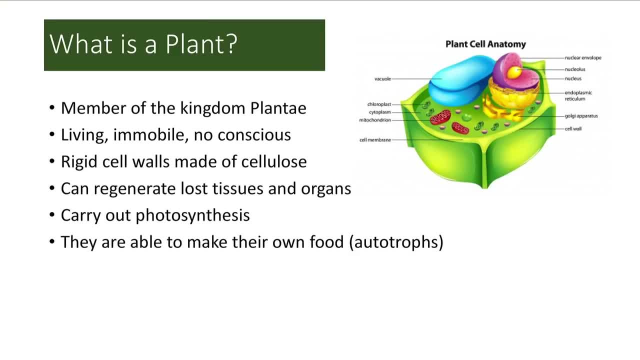 by the way that their seeds are able to move, But by themselves they can't move anywhere. They have no conscience, even though there are studies that say they react to things like music and talking and that type of thing. They're made up of multiple cells with rigid 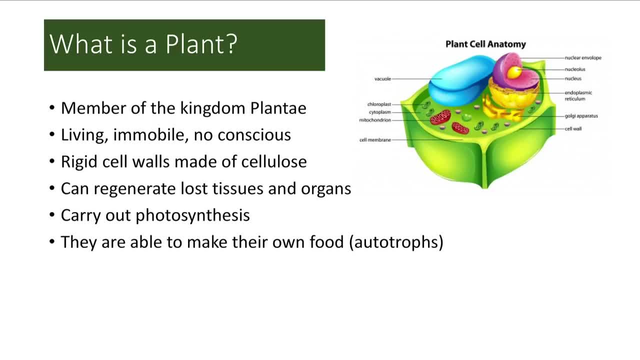 cell walls Made of cellulose. those cells are 90% water, which allows the things to move in between them, almost acting like sap in between. Generally, they can regenerate their lost tissues and organs. They carry out photosynthesis, which is a highly complex process that only they can do. And in that process of photosynthesis, 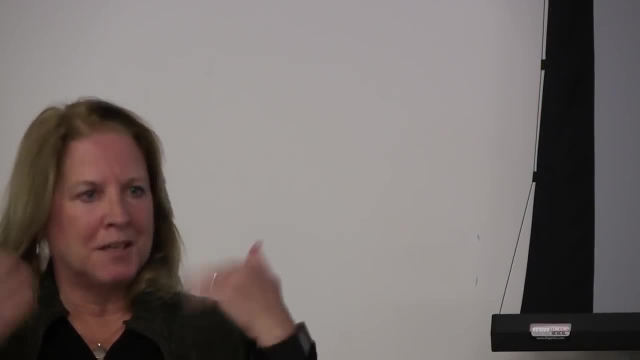 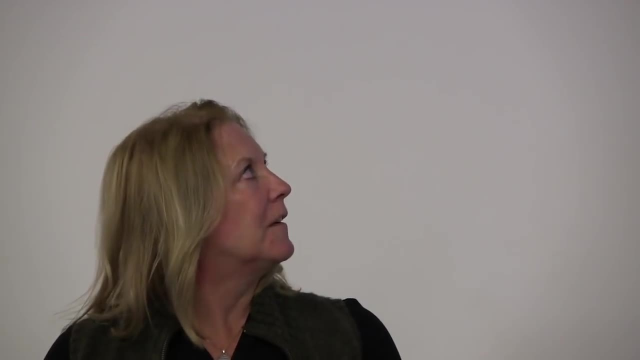 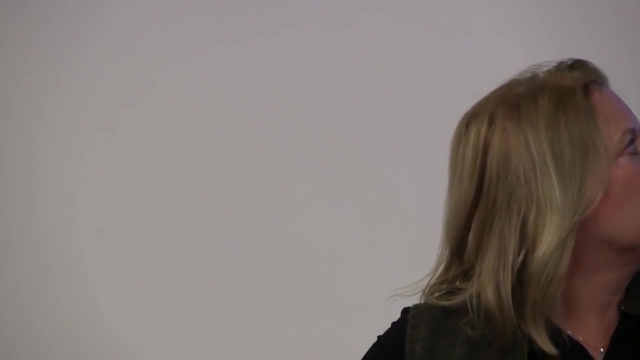 they're able to make their own food And we call that being autotrophs- filling their own troughs, almost you could say, versus man, we are heterotrophs. So yeah, Again looking back to Darwin's theory and this evolution of looking at plants and kind. 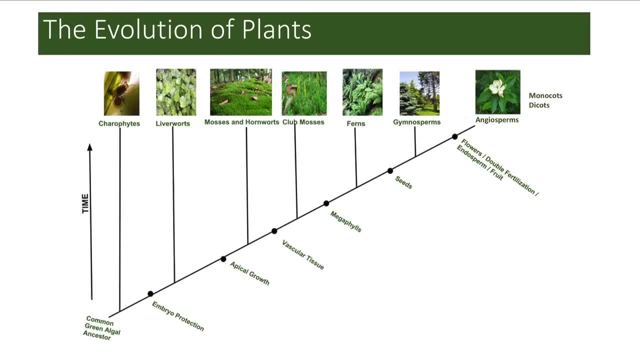 of where they started from. they all started from, basically, this common green algae ancestor. This was probably about 450 million years ago. starting way back there And a long time with evolution they developed things like one thing that was out of the box for them. 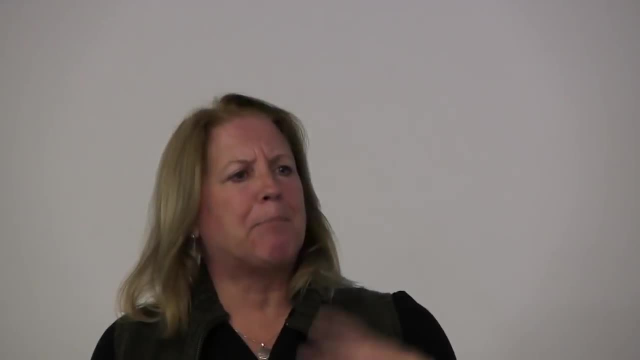 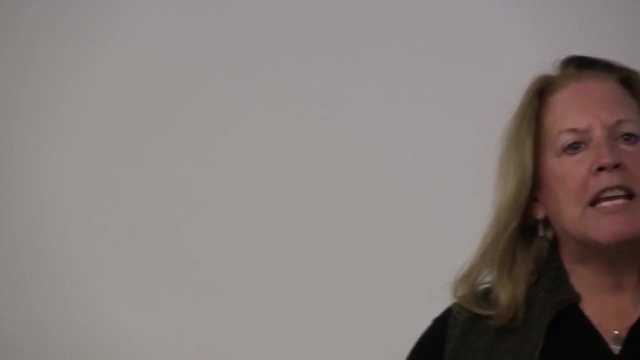 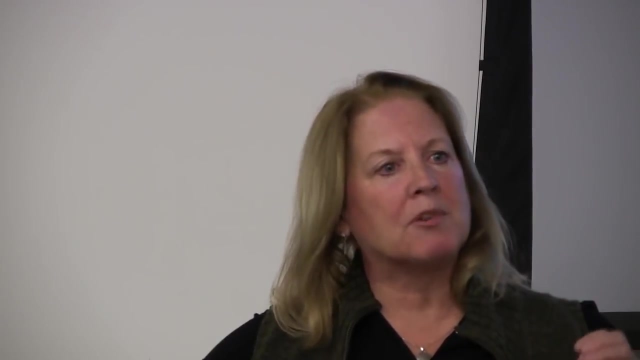 as they get into. about 400 million years ago they started to develop these spore-like structures that enabled them to kind of move, And those initial spore-like structures were, you know, needed to exist in a very wet environment And over time, with evolutionary process, they were able to develop these spores. 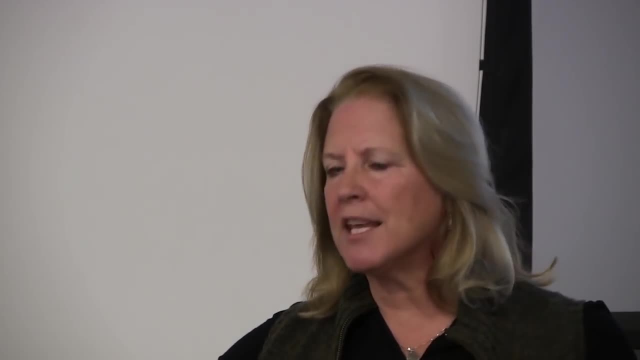 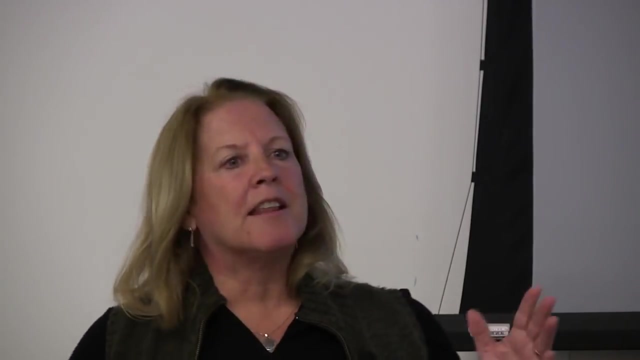 that were actually able to exist in a drier climate, Even though when we think of spore plants now, like our ferns and stuff like that, they typically exist in a more moist environment for Southern California. But even their ability to even move into those kind of environments and away from large bodies of water, really distinguish them. And so they start. they start, we start to see more and more species evolving. Eventually we get into, we get way up here into about 200 million years or about 250, into those gymnosperms. 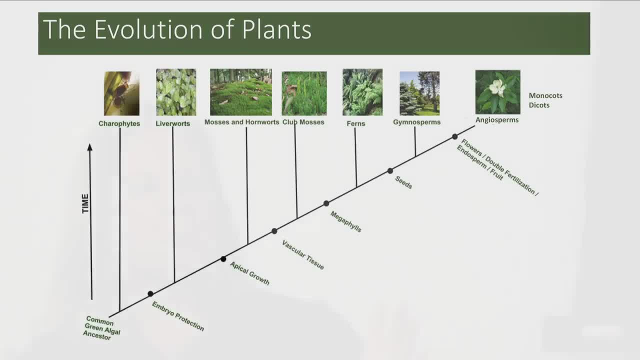 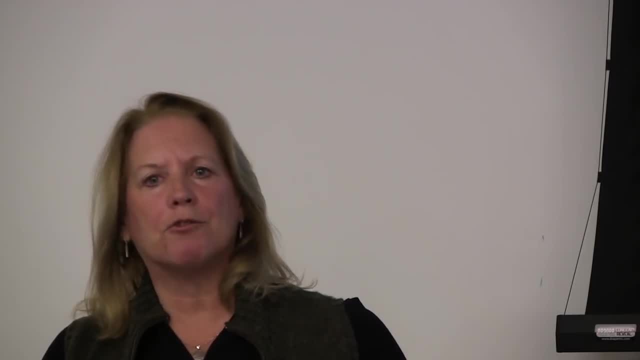 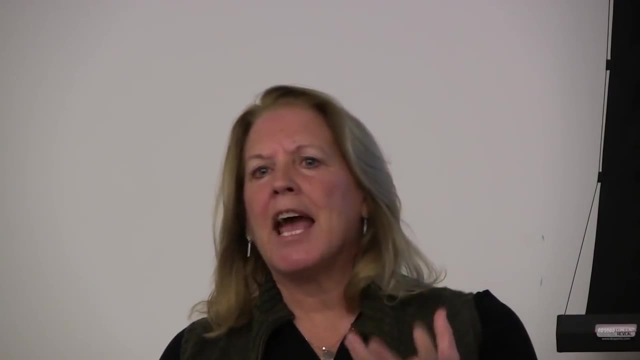 And those are. that's actually. we now see plants that are actually producing seed. It's highly evolutionary for them. The gymnosperms, which are your pines, your other conifers, your yews, your, I think, cycads, are even in here to a degree. They again, they have 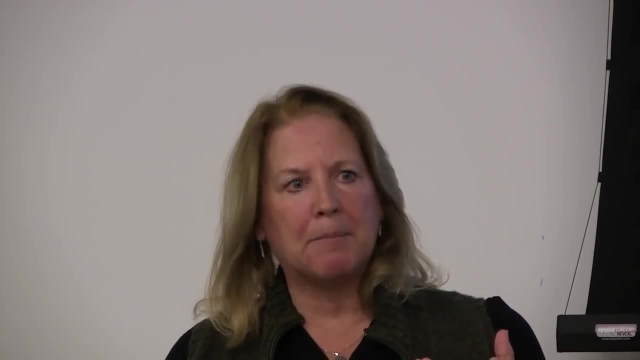 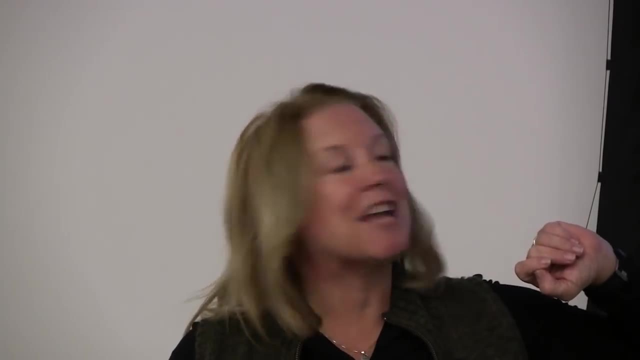 seeds, but those seeds are open so they can be easily pollinated by by the pollinator, Much more complex than they they are. the new kids on the block are the angiosperms, which means a covered seed. Those are our flowering plants, And I say flowering plants. 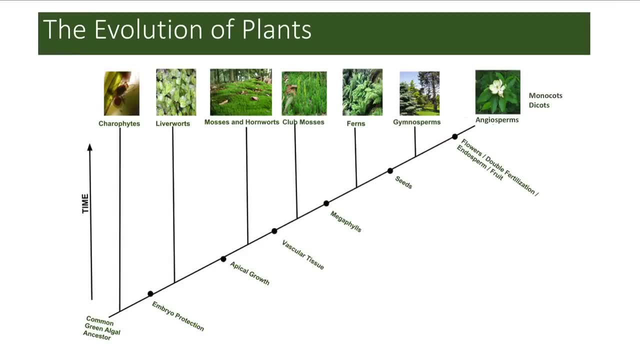 if they are called the flowering plant kingdom, but that includes almost all, like a lot of our broadleaf trees, our shrubs, things like that, that even though we don't see they're unlike the pines and that type of thing They do, they do a lot of the they do have. 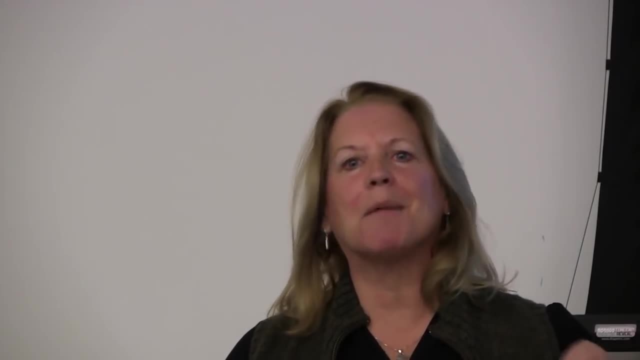 some, and that's what we call flammable plants. The more you see, the more you see that they're produce a seed that is covered, even though some of them, in the classic sense, we don't see them producing this big magnolia type of flower. but, and the 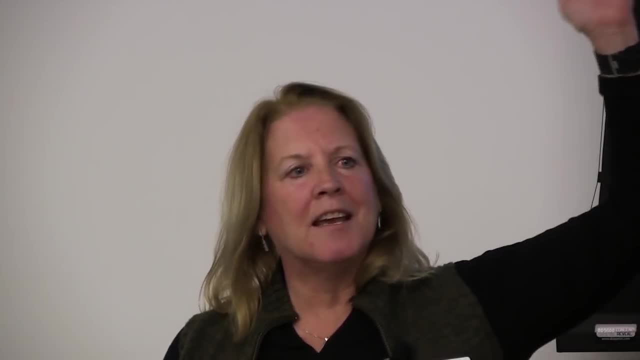 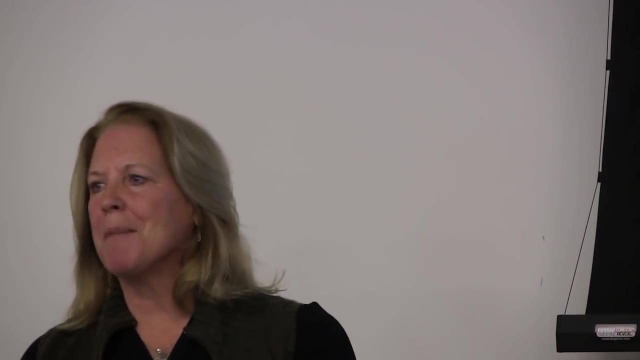 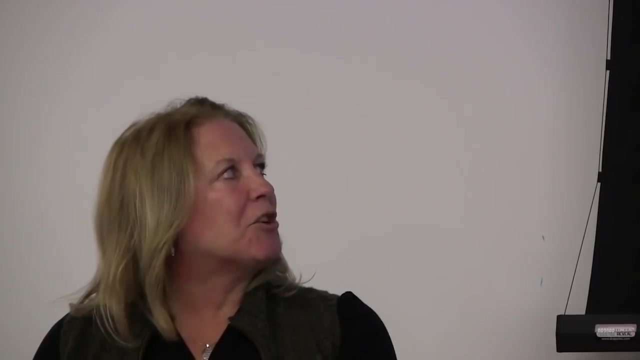 magnolia is probably speaking of. the magnolias is kind of the, the signature plant. that's one of the first flowering plants that is seen in that division. that's why, actually, the flower structure and the magnolia is really it's, it's really peculiar if you look at it in that angiosperm family we have there's. 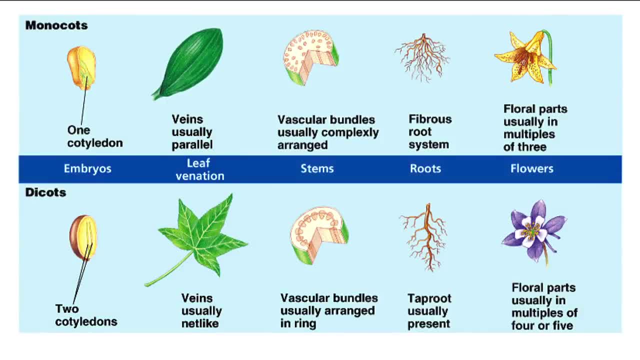 two types of plants we see in here, our monocots and our dicots. and again, why do we need to know some of this, where you know, we're kind of understanding how plants are kind of evolving and different things. so which are older, the monocots and the dicots? if the one thing that was always different to me is like: 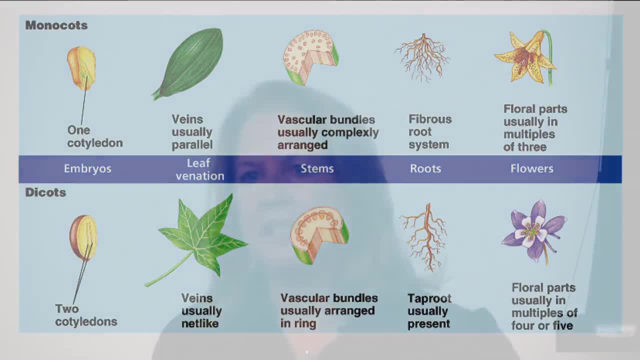 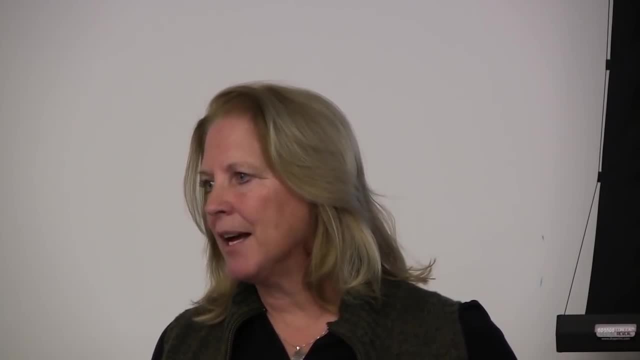 you know, you pick up a bag of weed and feed at your, at your local home center, and it's like I was always like how can I feed this to my lawn and have it killing these leaves while it's feeding something else? and that's kind of where. 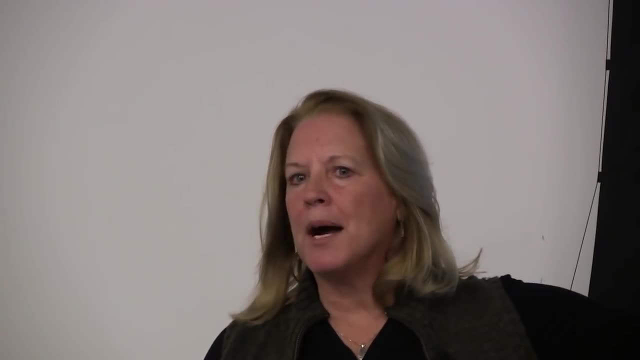 you're going to have to think about that and that's kind of where you're going to. you're going to have to think about that and that's kind of where you're going to. it's looking at that. that weed and feed you're buying is feeding the monocots. 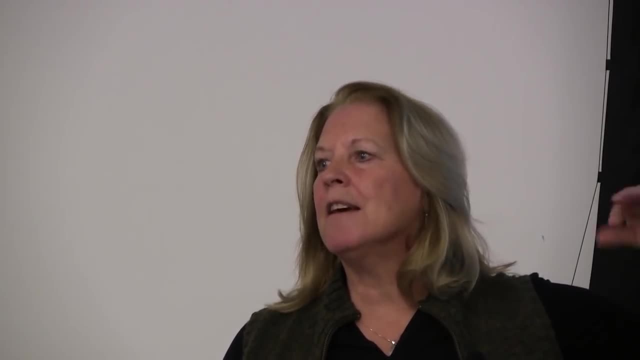 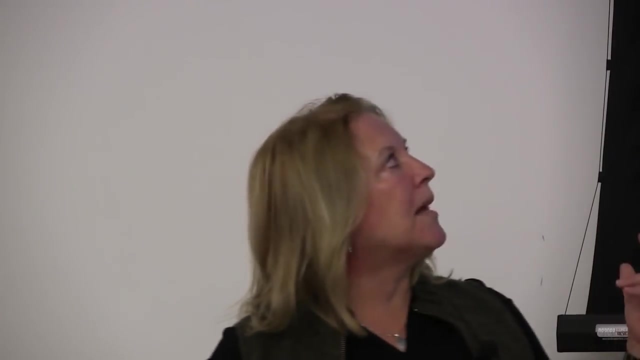 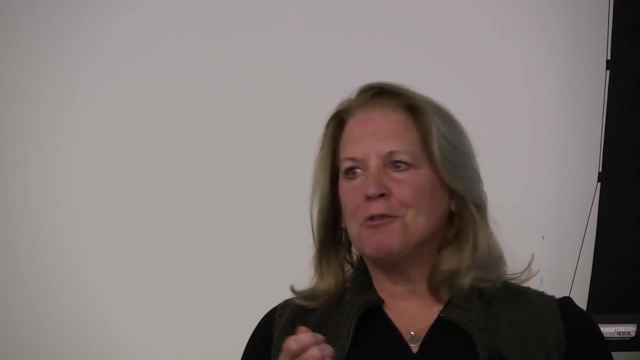 which are the, the grasses, and killing off the dicots, which are a lot of your broadleaf weeds, like your dandelion and so forth that exists in your lawn. so what makes them significant from each other is, you know, classically, when you were a kid and you put that, that bean seed- I don't know how many of you did. 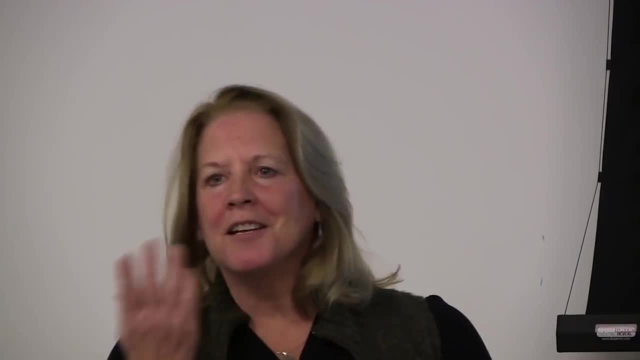 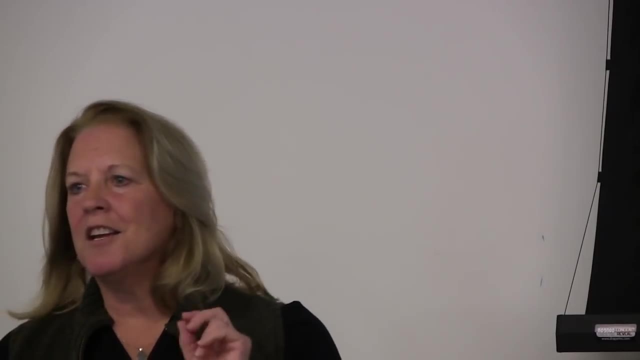 that between that wet napkin and came out a couple days later and you saw those two little seed leaves kind of coming forward. well, that was your classic. that bean plant is your classic dicot. it had two cotyledons. cotyledons are the seed leaves. you saw those seeds emerge. if you were to do, 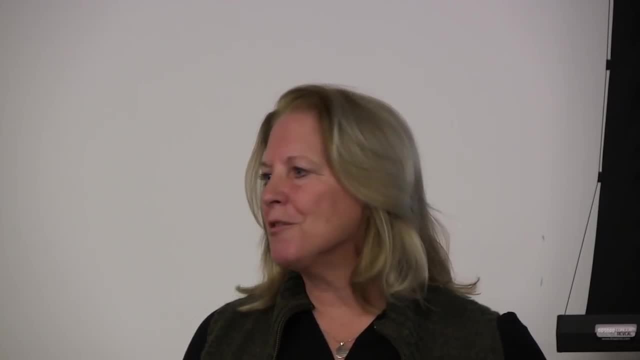 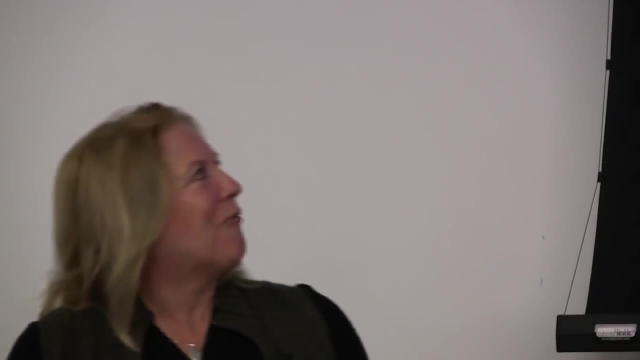 that with a grass seed or probably most of you working around your garden, you see those, those weedy palms and you see that one blade kind of coming up, but you don't get it right away is going to be get away from you really quickly, that is. 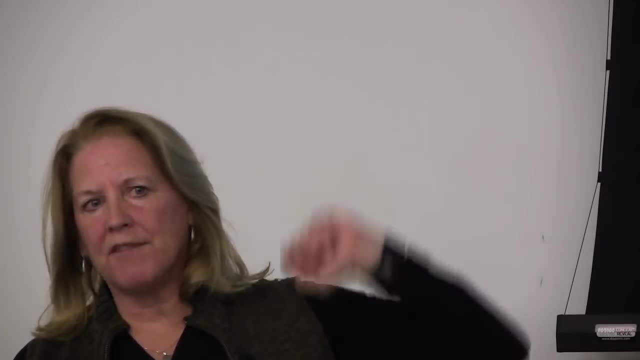 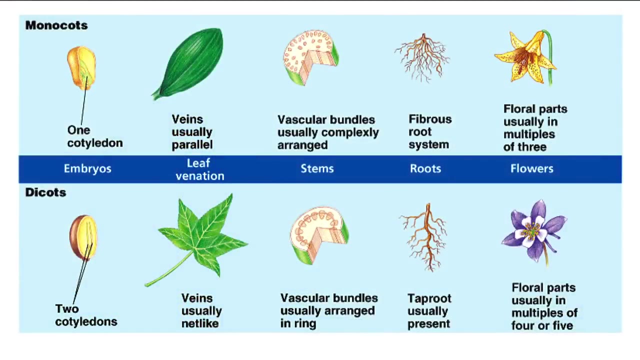 that's your classic monocot, those type of things. they have one seed leaf that comes out okay. there's also differences in the, in the leaves and that when you, when you typically if you see a leaf from either one of these divisions, your monocots, if you look at the leaves, that the veins of the and the leaves would. 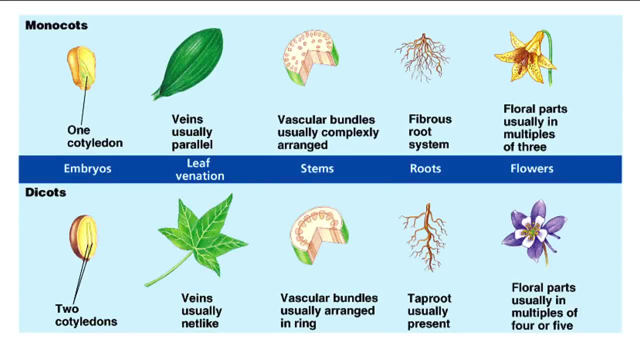 run parallel up the stems and you think of this a lot. when you look at your strappy plants, like your grasses or your agaves or your day lilies and flax and those type of things, you know you'll notice the leaves if you try to break it. 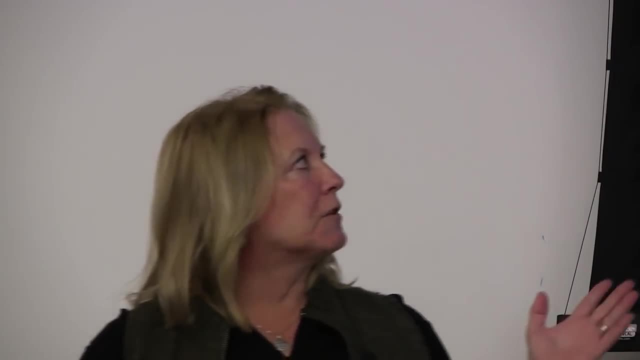 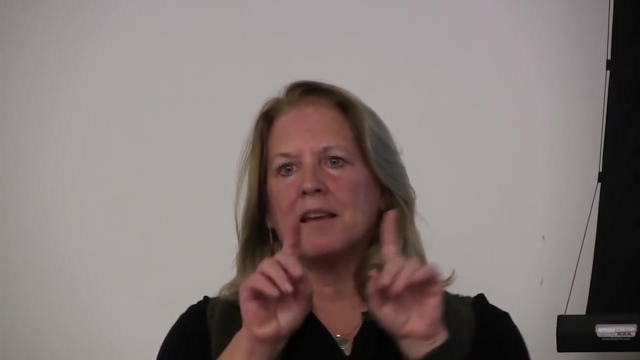 across the the, the veins are running parallel versus in the dicot family. the leaves are having net likes structure and there's a lot of different types of net like structures they have. but they, if you look at you, if you look at it, and I think you may be- 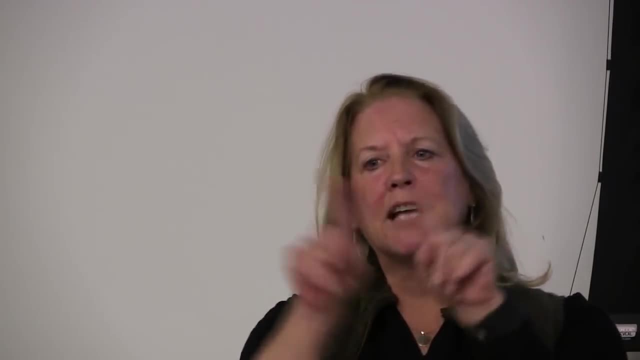 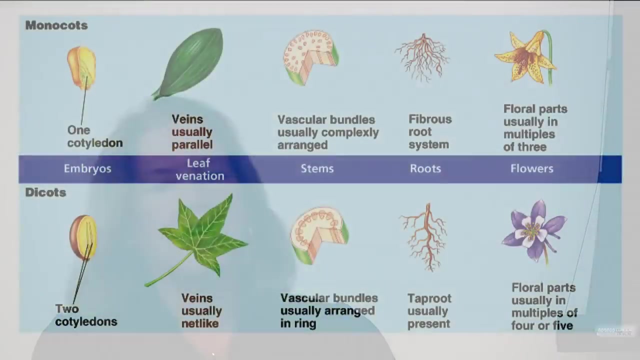 looking at some of this in your lab today. but you'll see the the veins kind of running running out across across the leaf. also, if I were to cut a stem in half of a of either one of those plants, I would notice in my monocots that the 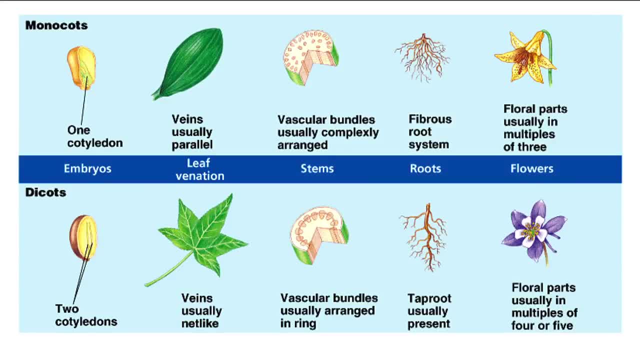 they're kind of scattered throughout the the little of the vascular bundles that I would see, those kind of scattered around. they fall in the periphery but they're. they're little scattered, scattered bundles, whereas when I look at my die pots they're all like in this nice. 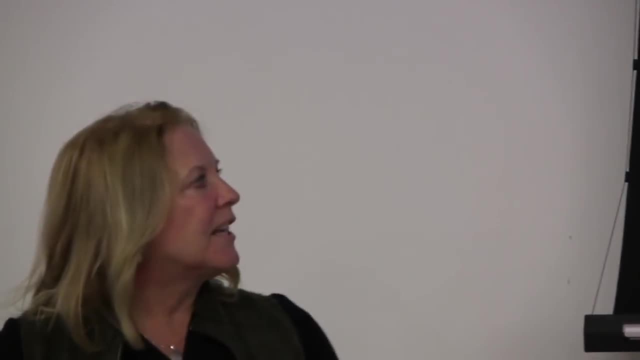 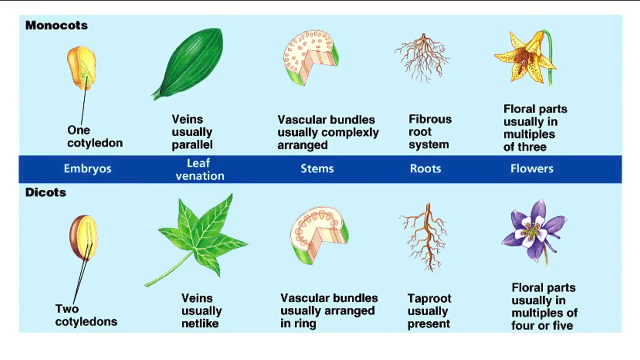 little neat little ring right in the plant. so I think I can tell that right away. again in the in the monocots my root system is a little bit different. their root systems are typically real fibrous. they don't have like a deep tap root. so you notice this again when you're out picking out your plants. you 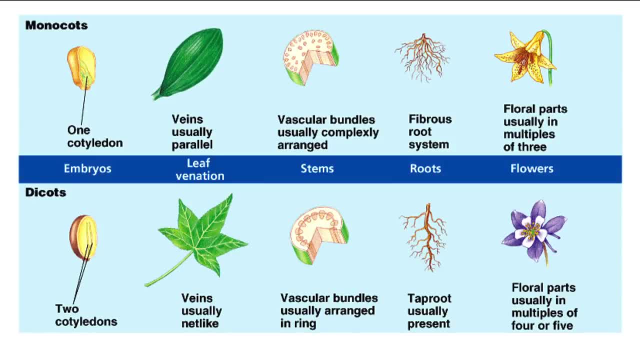 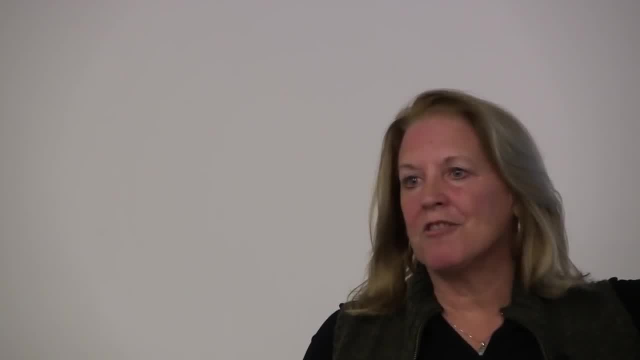 can kind of identify them. when you get those plants after the rain, you pull them out, you can see your your typically your monocots are fairly easy to get to those, those broadleaf weeds that you have in your yard. if you let them go for a while they can be really tough to conquer and to deal with, and the flower. 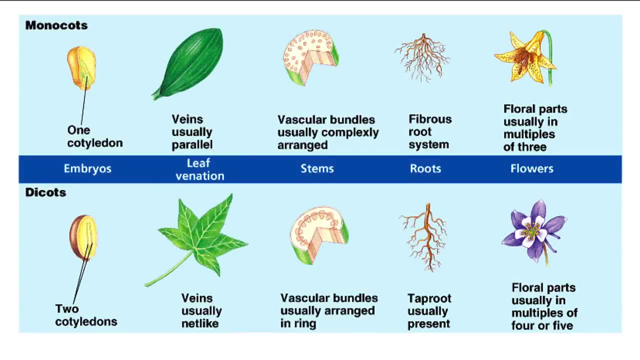 parts. unusually too, in the monocots. if I were to take apart a flower, I would see in the monocots that my flowers are typically in in groups of three. my petals, my plants, typically have three petals or six petals, sometimes nine, but they're in groups of three, and then in my dicots they're usually in multiples. 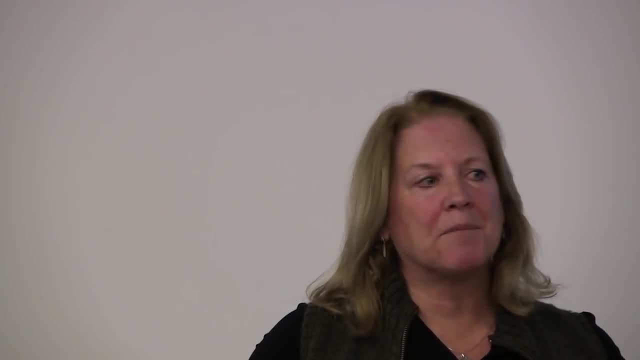 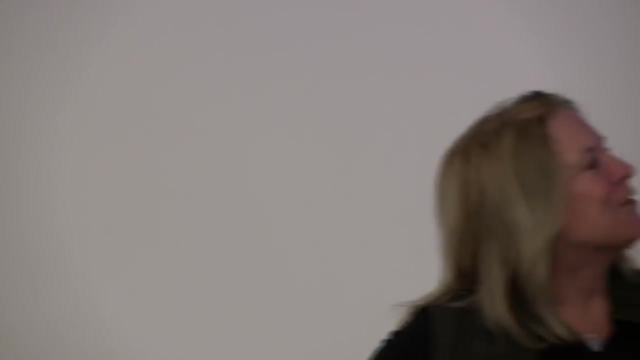 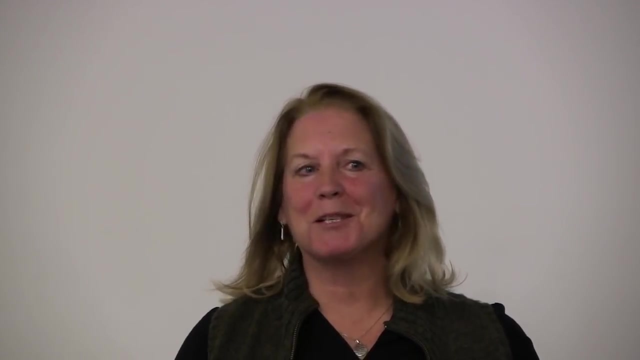 of four or five. so if you go out, you can kind of identify something fairly easily based on that. so so those are the kind of things that we are looking at, this and Mo is going to go on and talk to us about nomenclature botanic. 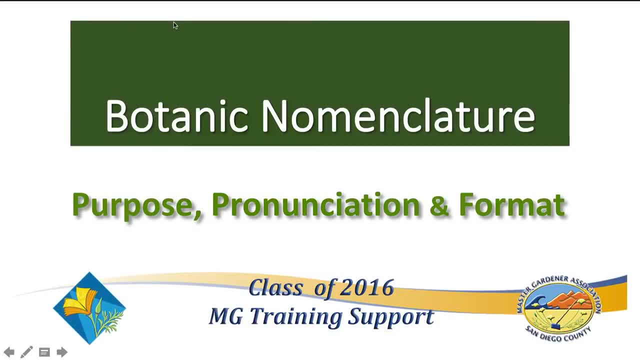 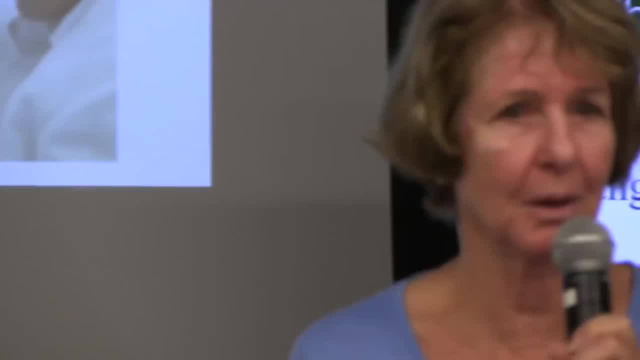 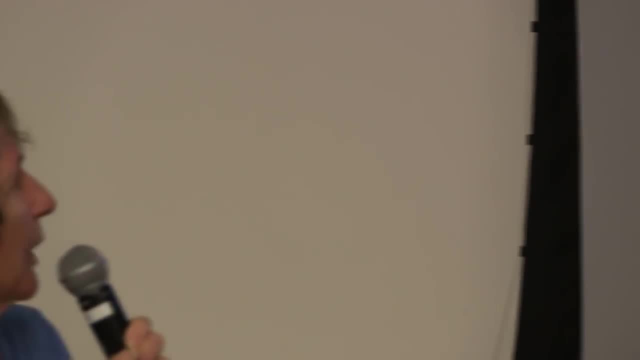 nomenclature. that's me. we are so lucky that Linnaeus discovered the system. if now we would have a terrible botanist, would have a terrible time explaining the their writings to people in other vernacular areas. so botanic you names are used: the. 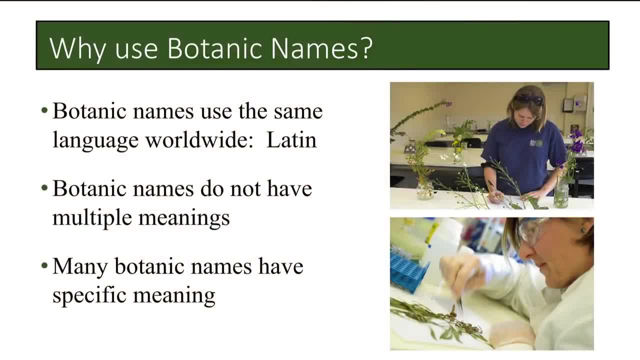 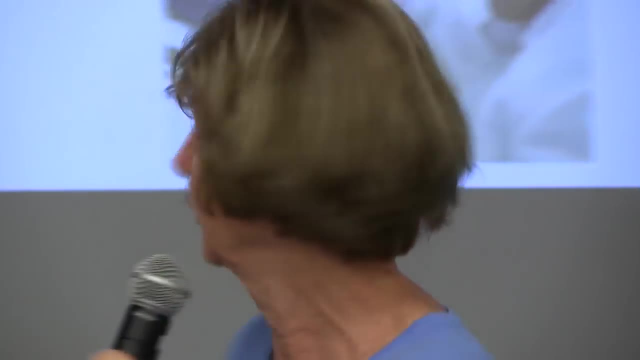 same use, the same language worldwide: Latin. so who else other than the Pope uses Latin, right? botanist, zoologists and many people in the medical profession, as Liz said, and both have botanic names, do not have multiple meanings, able to name references a specific plant and only one specific plant. many botanic, many. 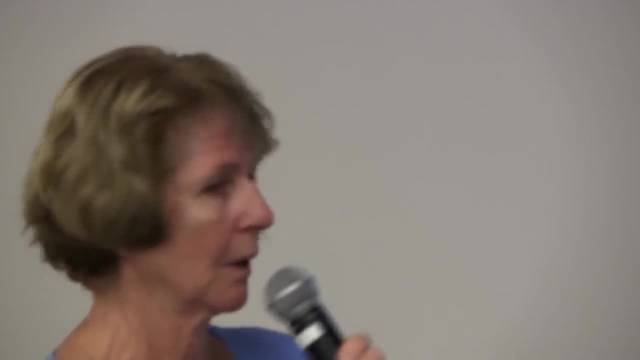 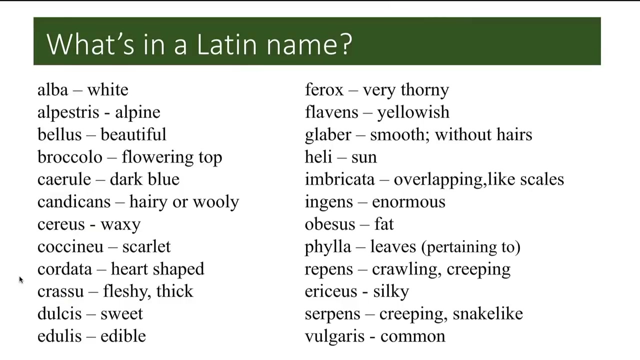 botanic names have specific meaning, such as what you see here. there are over 3,000 and you don't have to write all this down. there are over 3,000 Latin names, and here's just a little. look at them. say, you're in the nursery and you: 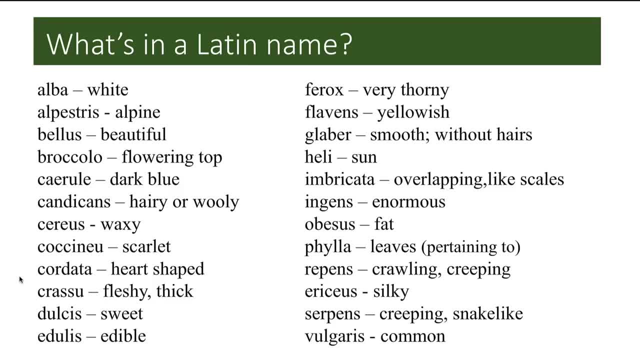 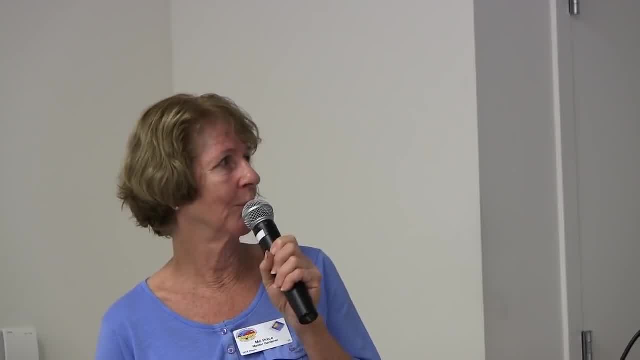 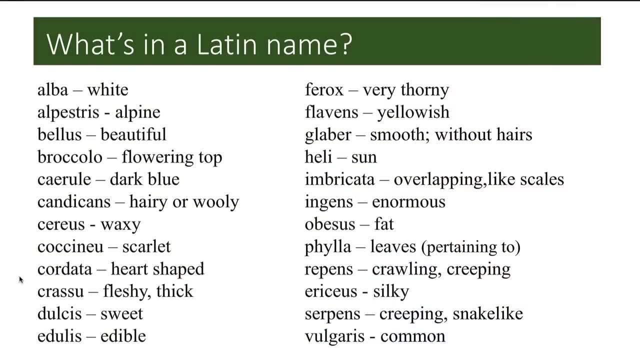 see a plant called a plumeria albis. what do you know about that plumeria? it darn better have a white flower. huh hey, is anyone hungry? see a plant and it's got a label on it. it says edulous- that means it's edible. you see a plant and it says something happens. you know that. 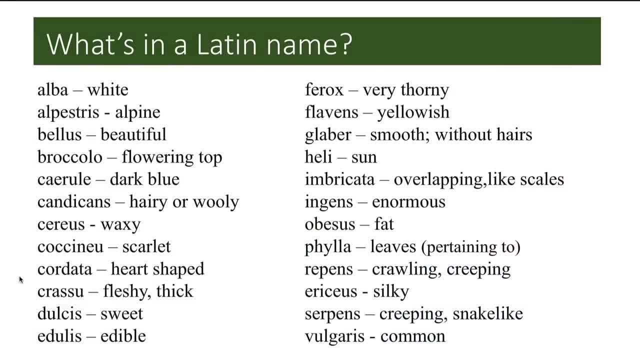 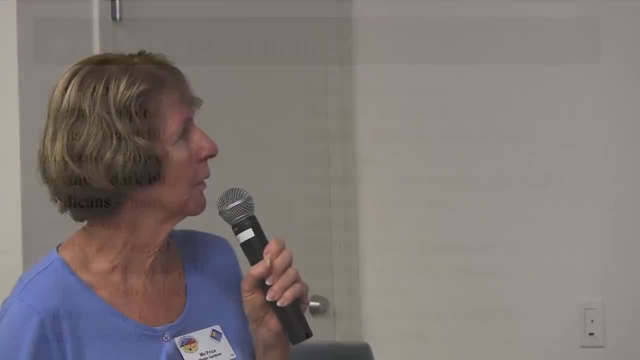 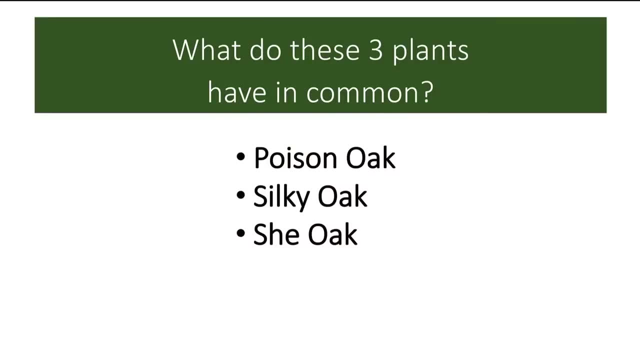 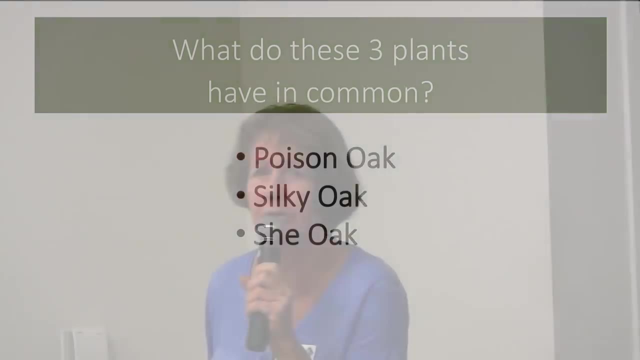 plant is going to be a creepy crawly plant. it is not going to be six feet tall. so what do these three plants have in common? any ideas? yell it out. what do they have in common? they're oaks. that's the answer. they're all oaks. yes, that's the 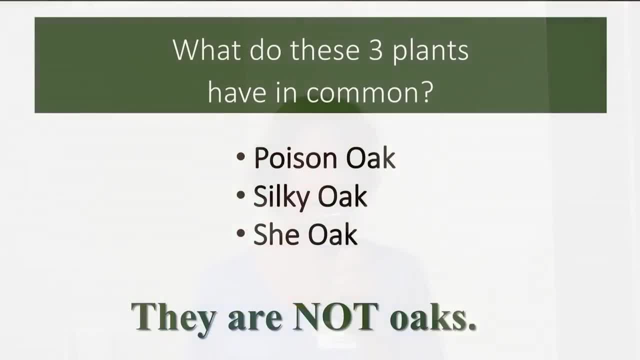 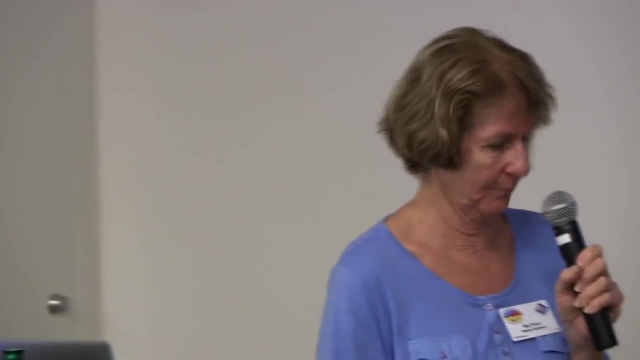 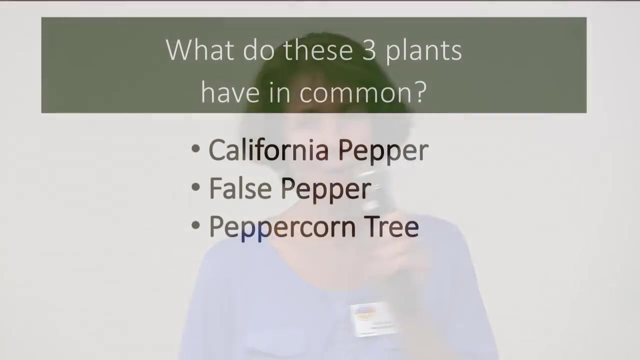 wrong answer. none of these plants are oaks. those are three common names: poison oak, silky oak and she oak- completely different families. they are not oaks by any stretch of the imagination, and that's part of the problem with using common names. want to try another one, you dare? what do these? 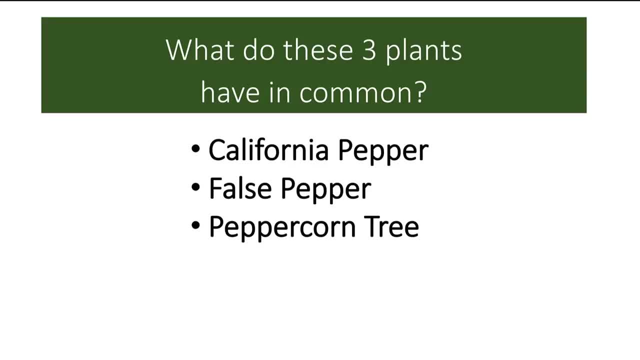 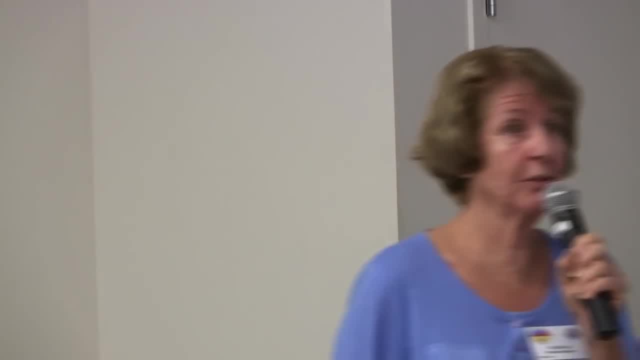 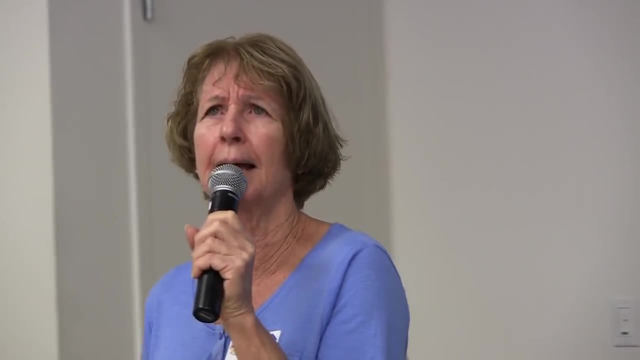 three plants have in common? well, they all have the name pepper in it. that's, that's true. they do anything else, they're all the same. that's good. that's the correct answer. yes, three different names, but all the same way. this call thisky nas Molly. something like I may be a little off on pronunciation, but they are all the same plant and they are native to Peru. I always thought the California pepper was native to California. I'm incorrect. so that's the problem with using common names, say they can be very misleading. the all these plants look like the California pepper. there's also a. 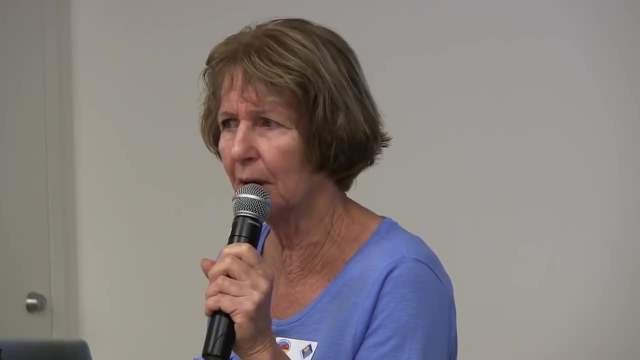 brazilian pepper. and now I'll go to the British. Which Brazilian do they have? what does it look like in texas? does it have an Atlantic laav doubt if there any Japanese구�na see a pepper? you see around town right now It's blooming like crazy. not blooming, it's. 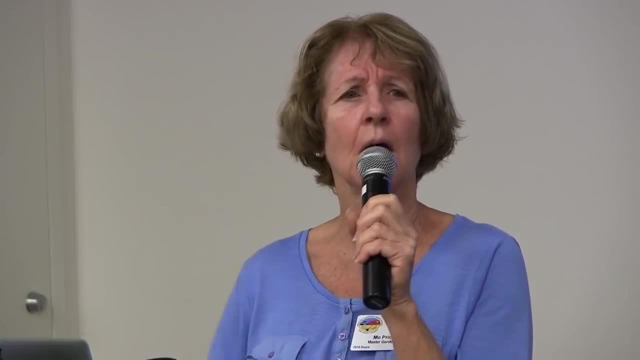 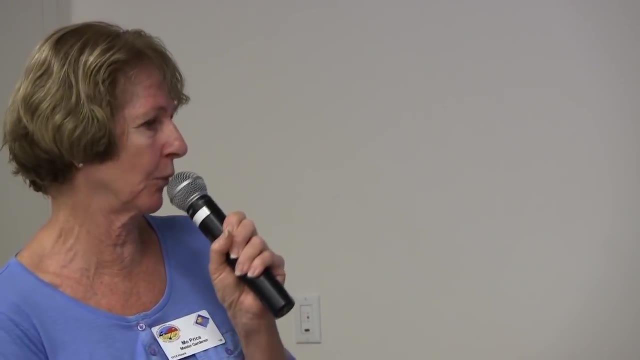 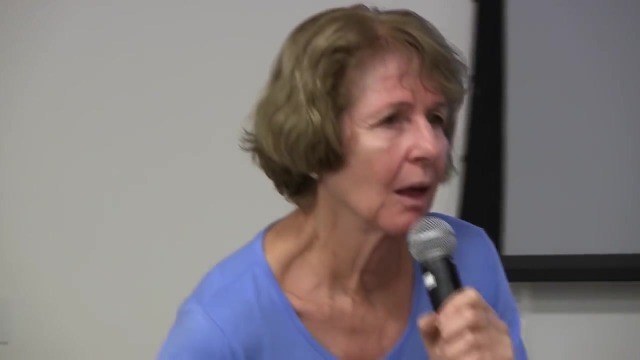 fruiting like crazy. It's got those tiny little red balls on it. Terribly invasive plant. Oh, she's going. yeah, it's a terribly invasive plant, as is this one. What's next? Pronunciation facts: Probably the biggest reason why people do. 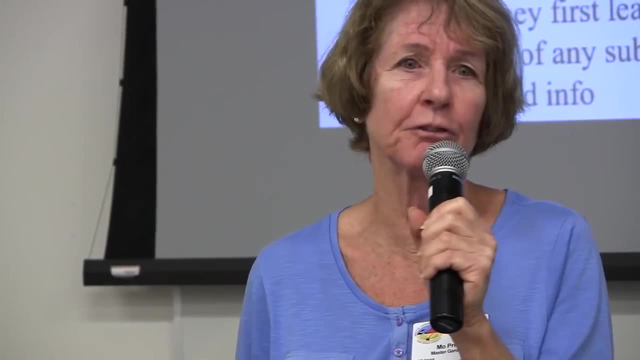 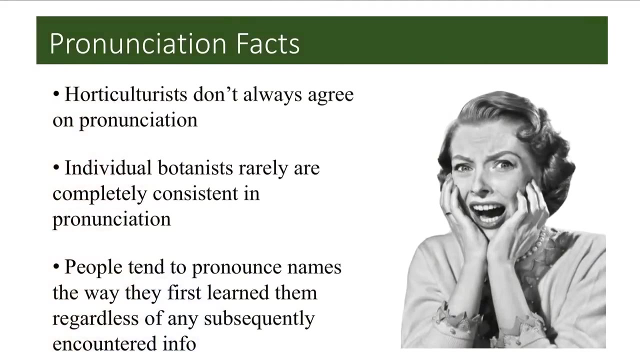 not want to use botanic names is because they're afraid they are going to mispronounce the botanic name. But take heart, horticulturists don't always agree on pronunciation. Individual botanists rarely are completely consistent in pronunciation and people tend to pronounce names the way they. 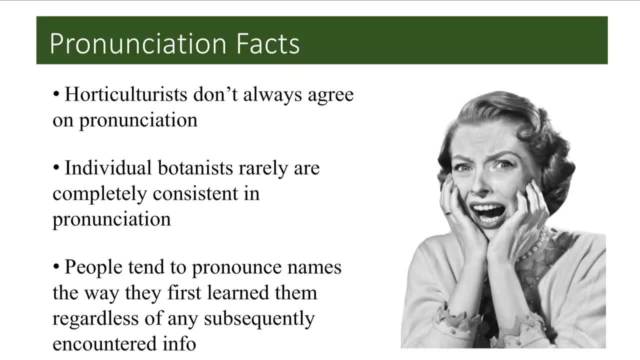 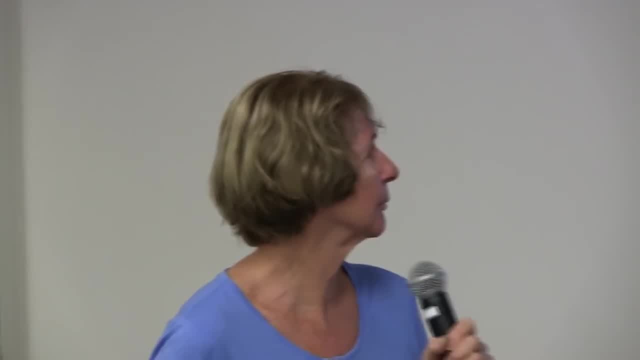 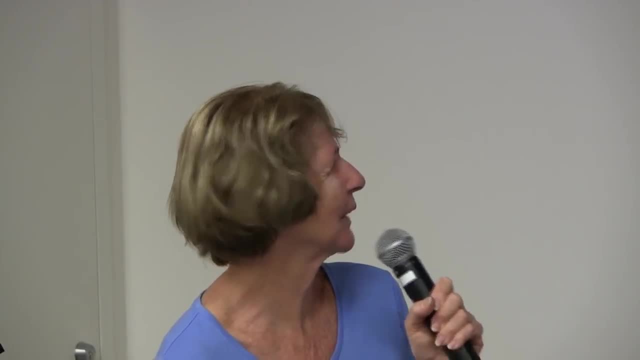 first learned them regardless of any subsequently encountered information. So don't worry about not being able to pronounce a botanic name. Isn't she cute? Liz, put her in there for me. Okay, look at this name. Kind of a big one, isn't it? A? 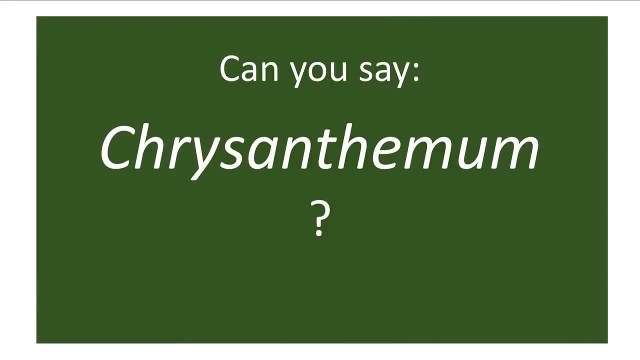 long name. If you didn't know it, you would think it might be rather daunting. How would you say that name if you're just looking at it for the first time? Would you say I can't say that right. Kind of scary, isn't it? 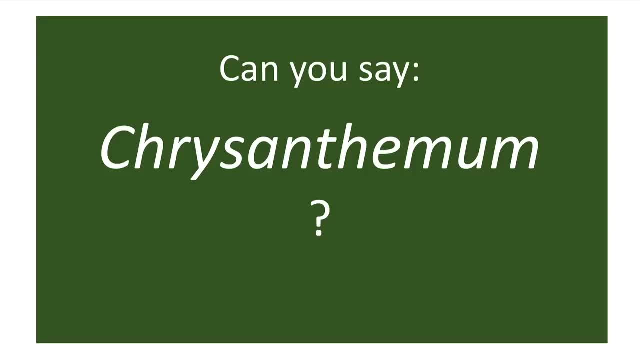 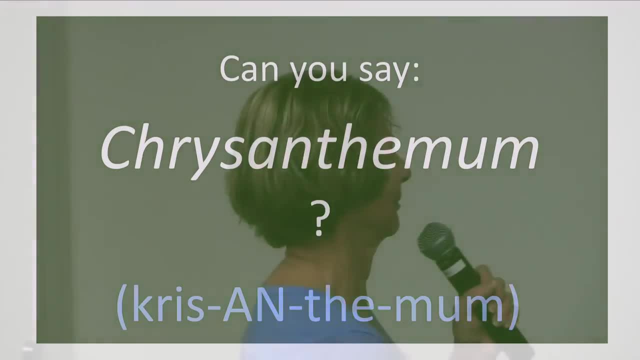 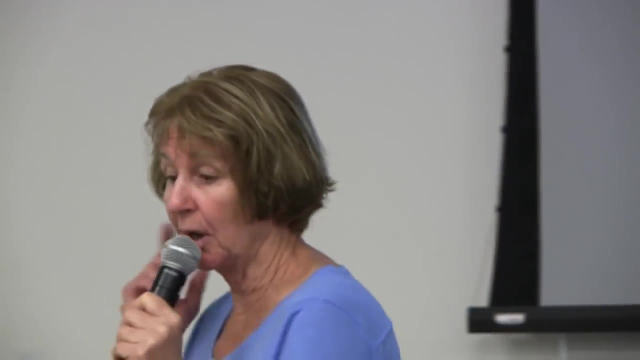 Well, I bet we can all say it right. Can anyone say it? Pretty easy, isn't it? It's a botanic name, but it's easy. So let's talk a little bit about botanic name pronunciation. I will first say I don't know any website you can go to. 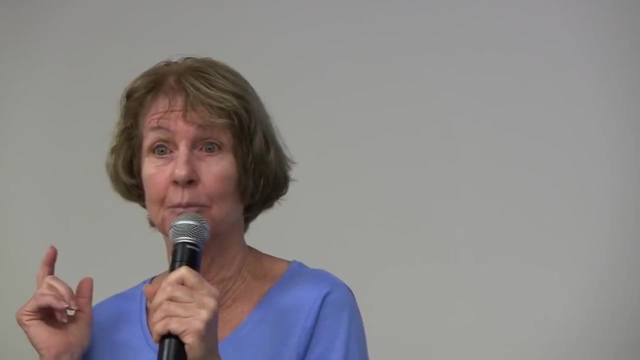 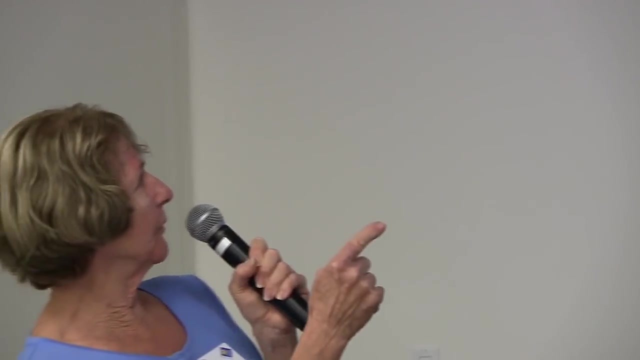 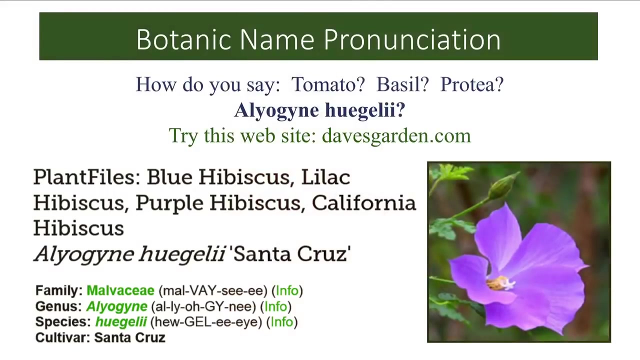 where someone will actually rattle off a botanic name for you: Chrysanthemum, Chrysanthemum. It won't happen. However, if you look at this, how do you say that first one: Tomato, Tomato. Ah, she says, you said tomato, I say tomato. How about the next one? 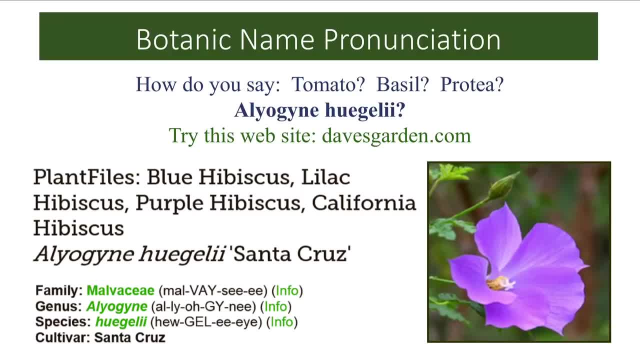 Basil. Ah, is that you again? What part of the country are you from? She's from California. She says basil, I say basil. And the last one, Lorene, I'll ask you because you know about these plants: How do you say that one Protea, Protea. Sometimes I say: 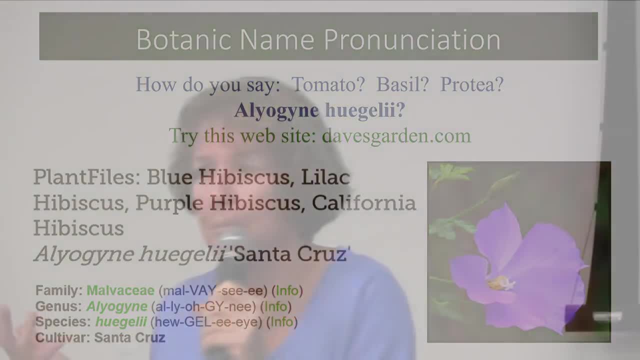 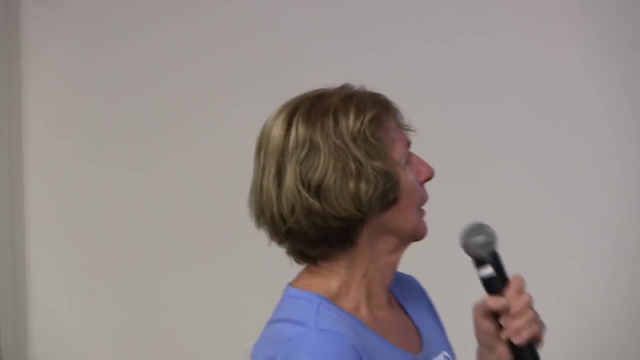 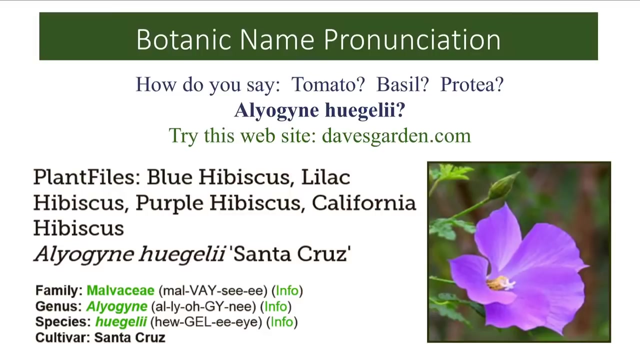 protea. Sometimes I say protea, It doesn't matter. Say what Protea, Protea, It doesn't matter, They're all good, The next one. You don't have to try this one right now, but that really is a little intimidating, isn't it? So there is help. There is help. 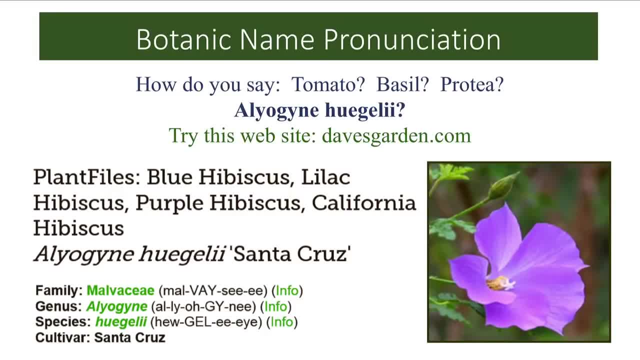 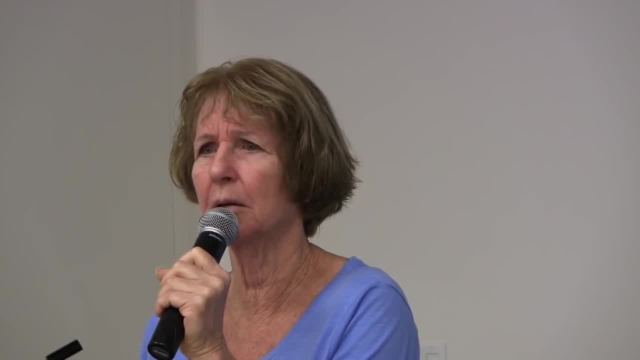 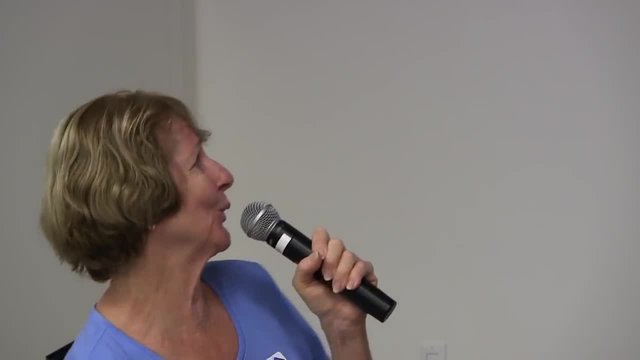 Try this website. How many use davesgardencom? A few of you, By the way. how many of you use botanic names regularly? Not you, Not staff, You don't count, Some of you do. Okay, This website is very helpful. 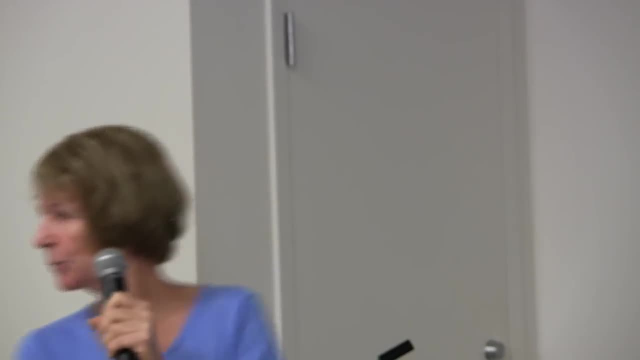 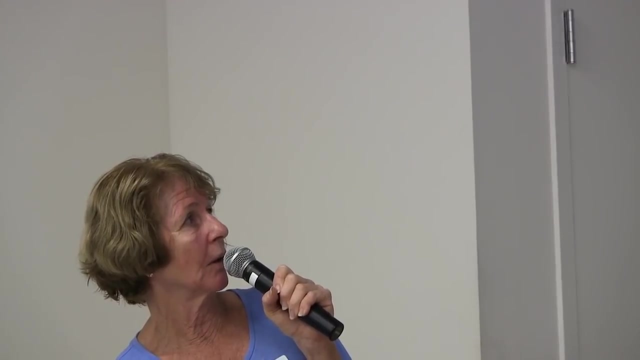 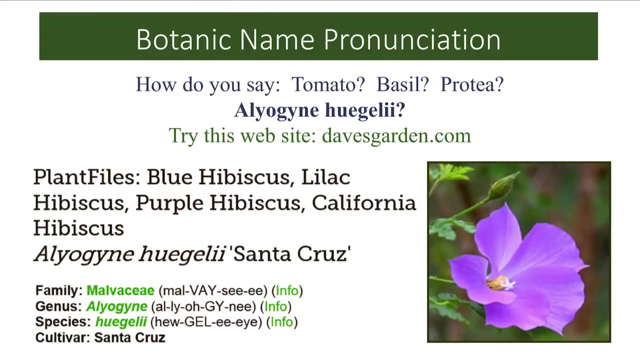 davesgardencom and this little, this little thing here. this is a screen print, So the first thing you learn from davesgardencom is this particular plant, and I'll pronounce it aliogonyhugeliae- Pretty easy. once you say it a couple of times, It's even kind of 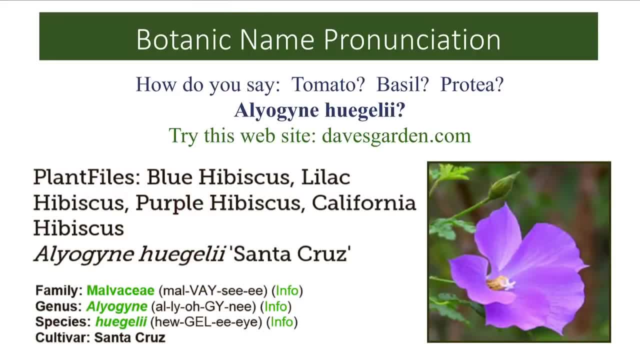 fun, It rolls off your tongue. plant Aliogony hugulii. It's got four common names: blue hibiscus, lila hibiscus, purple hibiscus and California hibiscus. Oh my, So you pronounce it Aliogony. 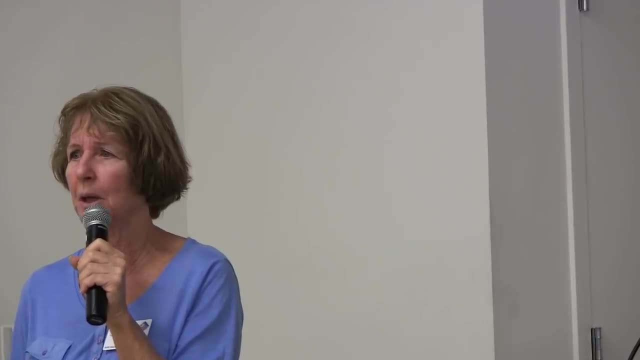 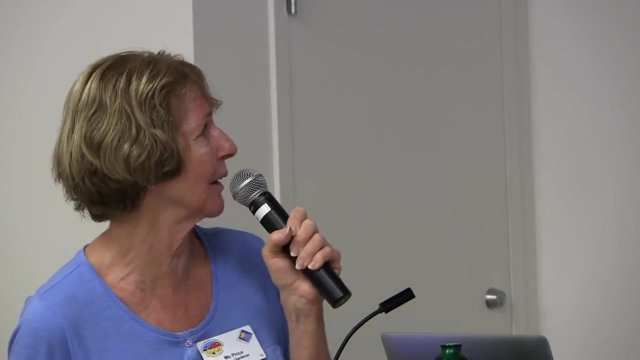 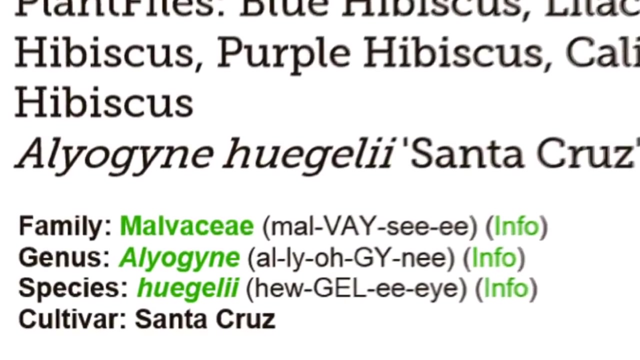 hugulii And what is down below. It's in the family, Someone who got the family. someone picked this family today for her plant and she didn't know how to say it. It's right here. Melvaceae- Pretty easy, The genus. you've got the. 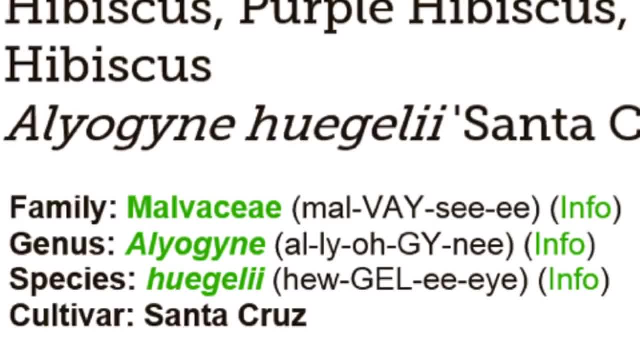 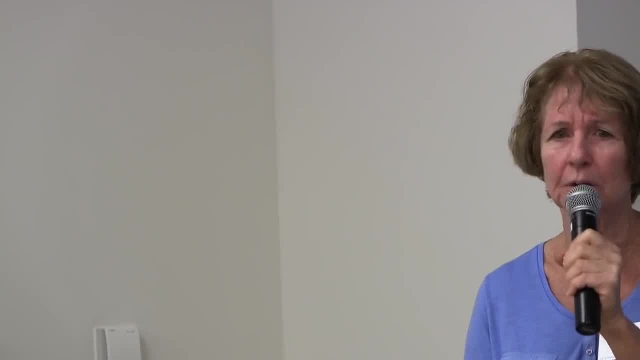 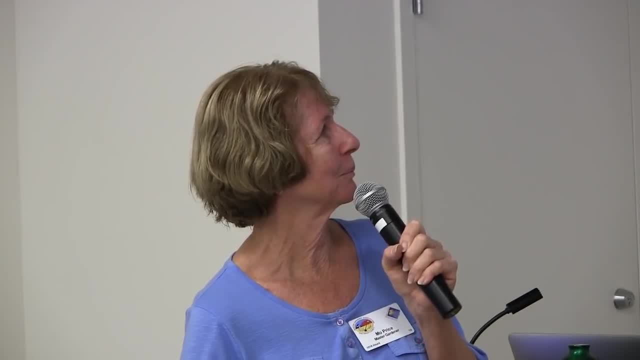 pronunciation: Aliogony and the species hugulii. So use this website. It's very easy. It really makes it easy for you to learn how to pronounce botanic names. I know I use it all the time. So Liz talked a little bit. 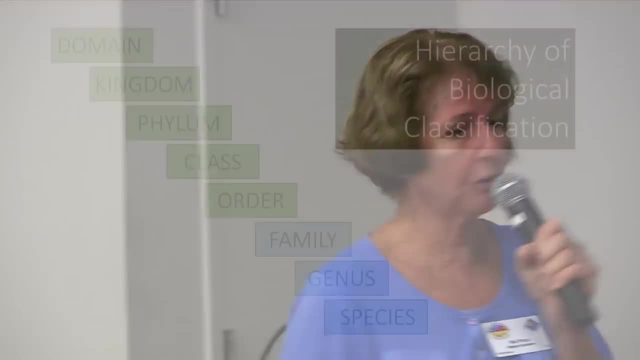 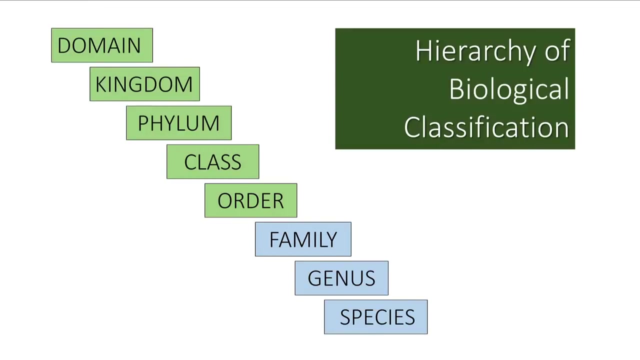 about the higher hierarchy of biological classification. But to be honest with you, these things in green I never use them. Sorry, Liz, I never use them, But I do use the bottom three: The family, the genus and the species. The genus and the species are probably the two most important. 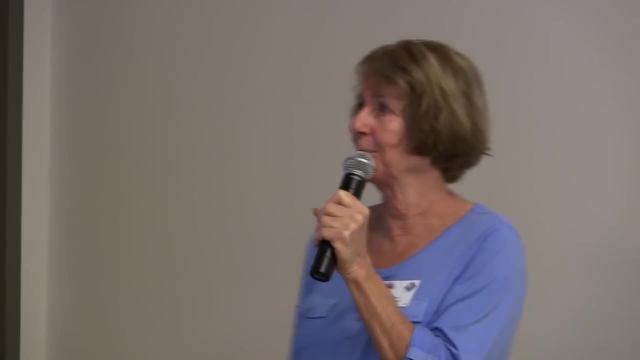 items, but the family has a lot of importance as well, So the purpose of this slide is to help you understand the hierarchy of biological classification, So the family, the genus and the species hugulii. The genus and the species are probably the two most 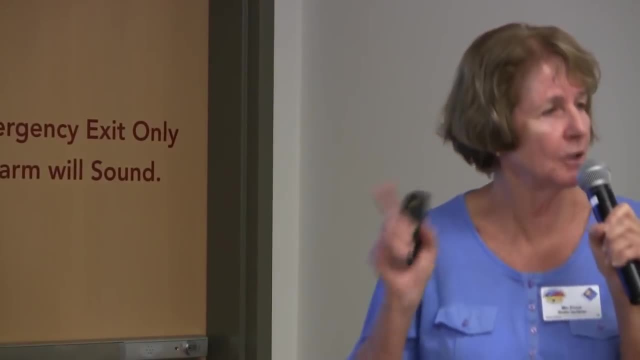 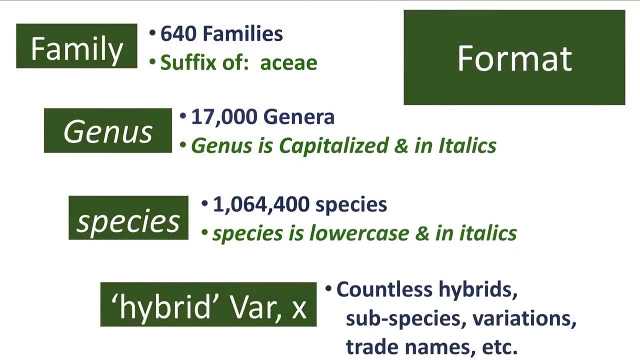 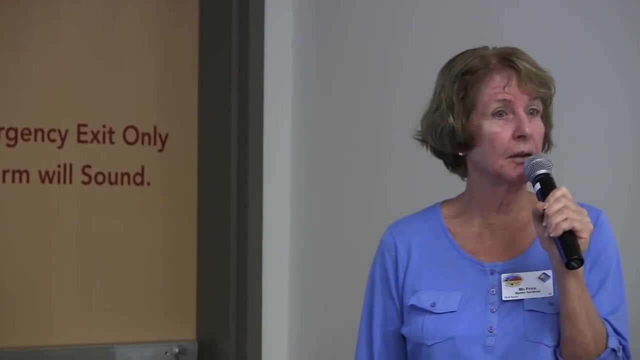 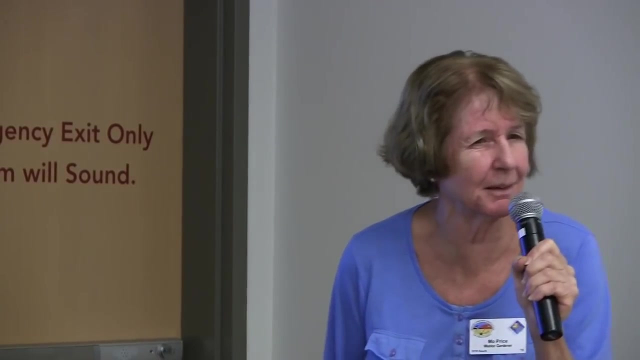 is merely to tell you, to show you how to read and to write a botanic name. so it's called format. so the first thing we have is the family. there are over 600 different families of plants and they all end in the suffix a, CEA, e. you may see. thank you, they didn't know this. this didn't always. happen. I'd say maybe 15, 20 years ago there were some plants that didn't end in the suffix, but now they do. a CEA e, the genus is a lower order of family and there are over 17,000 genera. and when, When you're writing, it's very important to capitalize the genus and write it in italics. 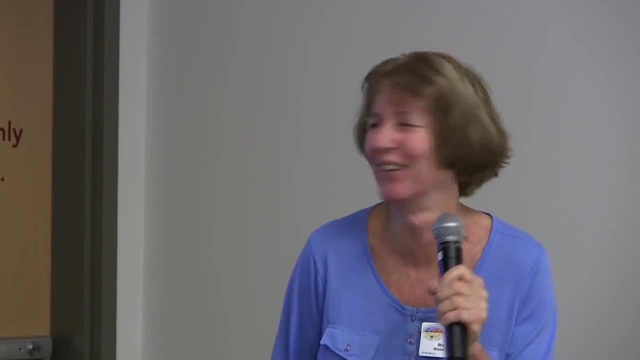 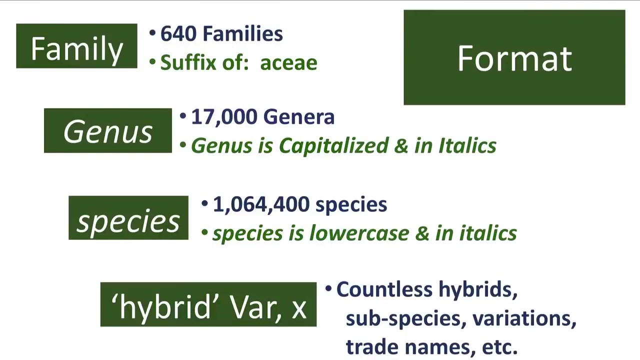 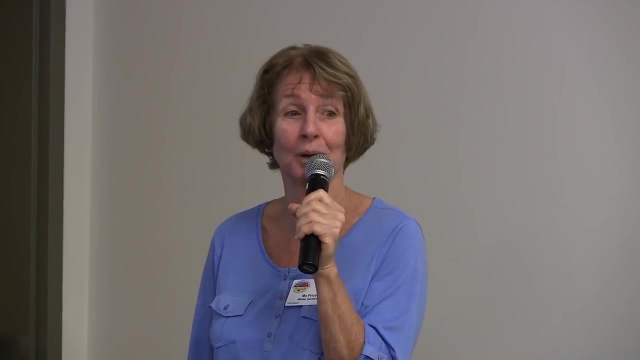 The attorney is looking at me like: are you crazy? Next we have the species, and there are over a million different species. The species is always in lowercase and in italics. I see a lot of people writing: If you didn't print the PowerPoint, you can go back and print it. it might be very helpful. 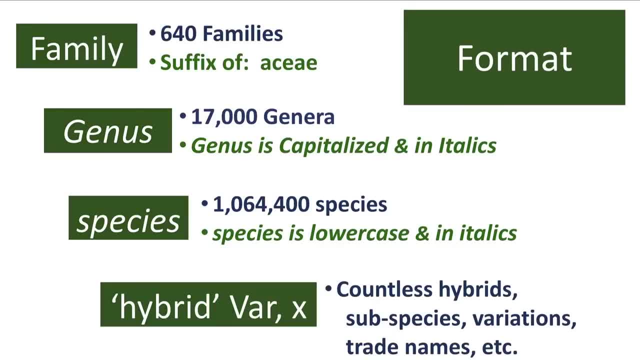 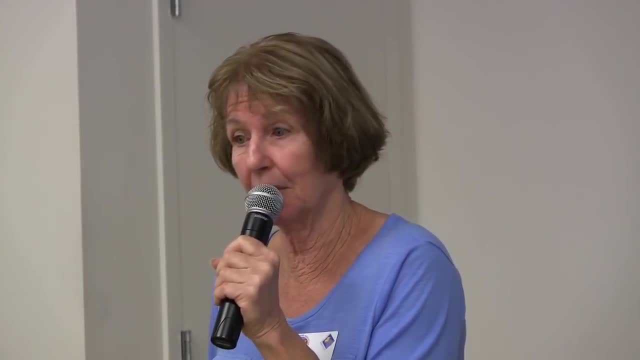 The last thing is: after species, there's a further breakdown and you've got lots of different things here. You've got hybrids, you've got subspecies, you've got variations, you've got trade names, and if you read your handbook- which I'm sure you did- they talk about all of these different 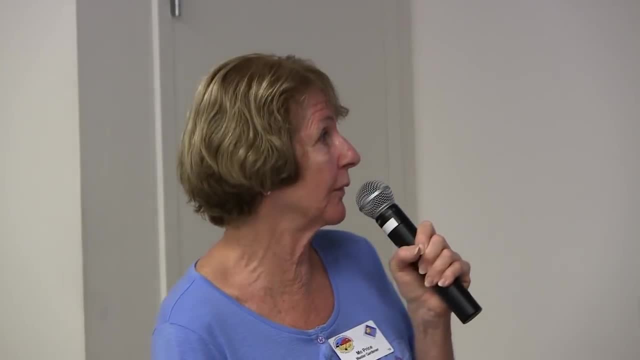 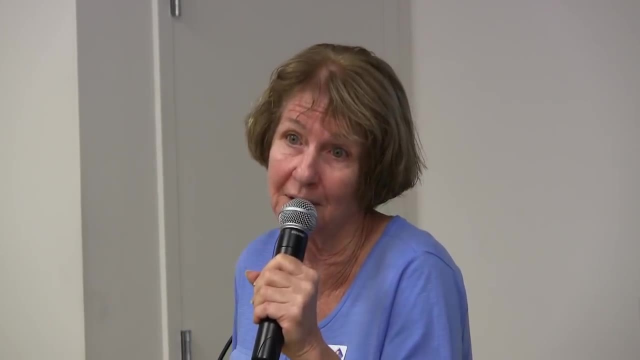 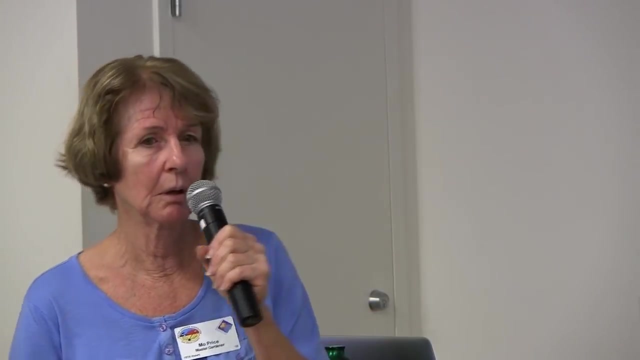 things. Actually, I don't concern myself. I don't concern myself with these things because I'm not creating hybrids. I'm not creating new hybrids. I don't know how to have to write them, but I do read them. The one thing you might want to consider is: if a plant has a hybrid, it is there for a. particular reason- and I think this was covered in the manual- like they made otherwise maybe not so pretty- flower prettier colors. sometimes they put something on a different root stock to make it stronger. In that case it might have a hybrid after it. 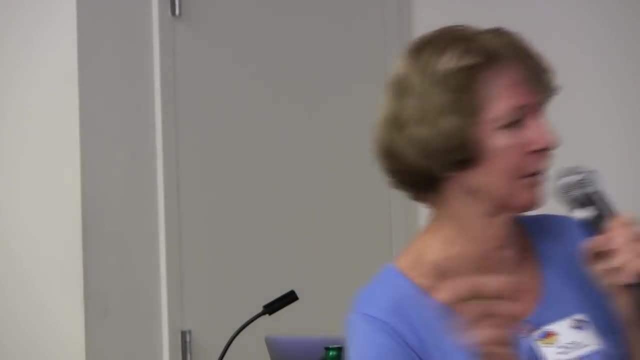 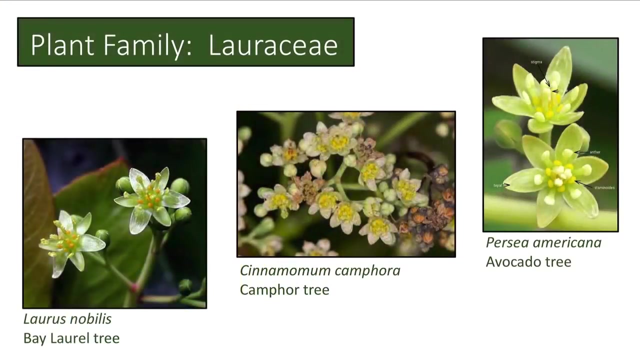 Or someone may find one out in the field. well, never mind, that's not quite it, let's keep going. So let's look at an example. This is a plant family, the Lauraceae family, and it's really funny because these flowers. 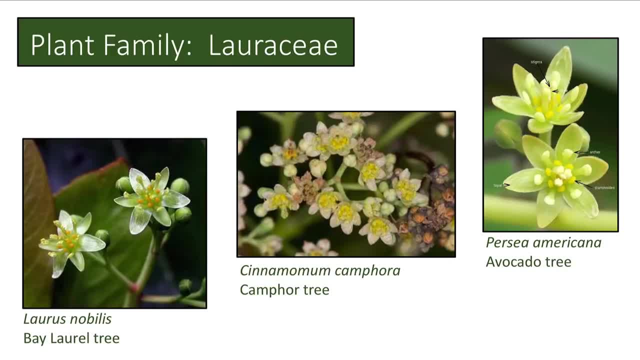 all look alike, don't they? But they are really three very different looking plants. One of them has a flower, Two of them has a plant. The flowers here are from a bay laurel tree, The flowers here are from a camphor tree and the flowers here are from an avocado tree. 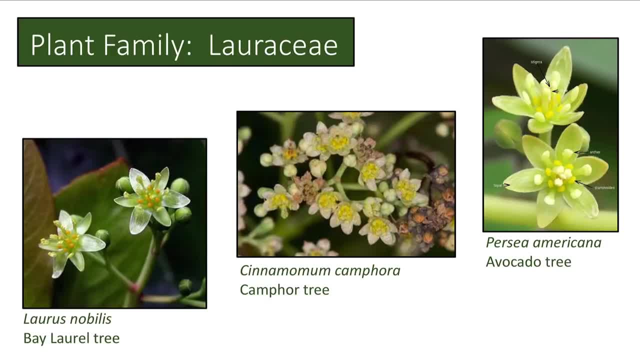 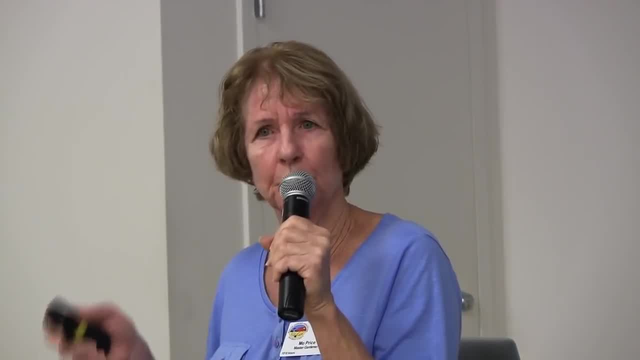 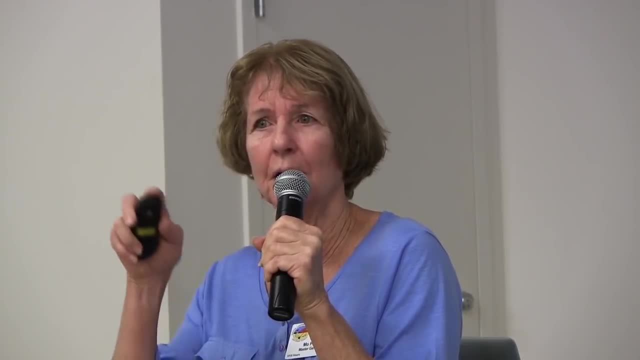 And when botanists are grouping plants in families, the first thing they look at is the flower, And plant families are typically grouped by flower. And why is this? It's because when you go from the flower, we talk about reproduction and the reproductive. 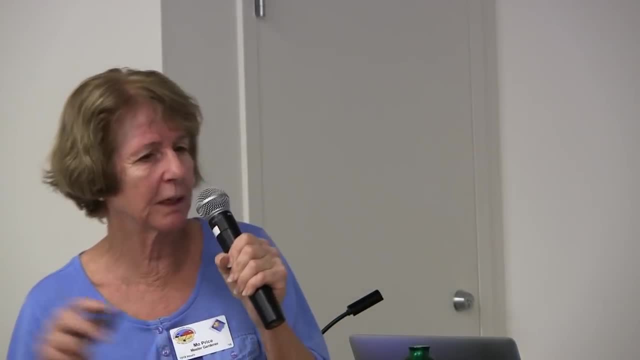 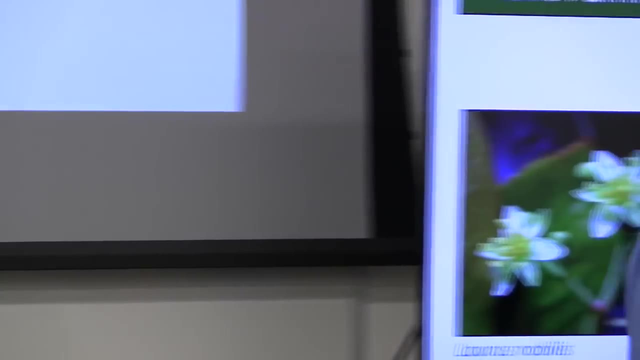 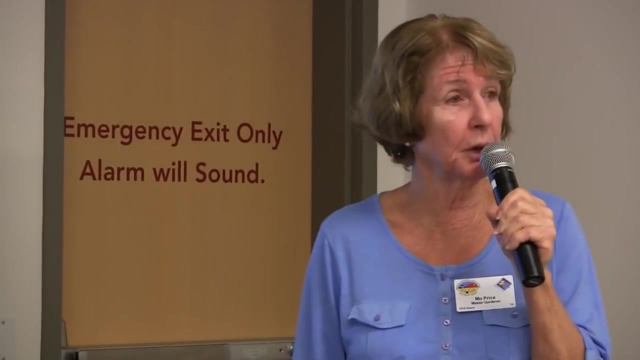 organs in these flowers. These flowers are very similar, which kind of links them to the family. So why would you care about the family? If you know a family name, what does it matter? Well, I grow proteas and if I get a seed, a protea seed, and I want to start it, I know. 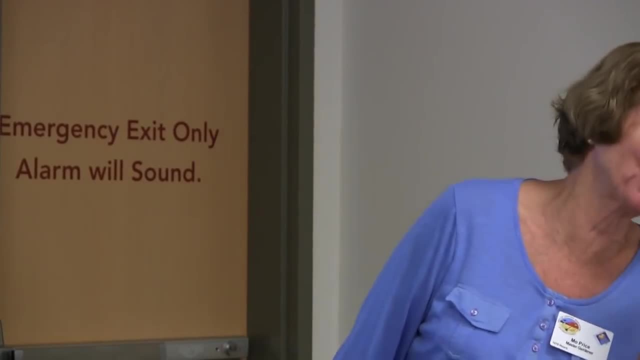 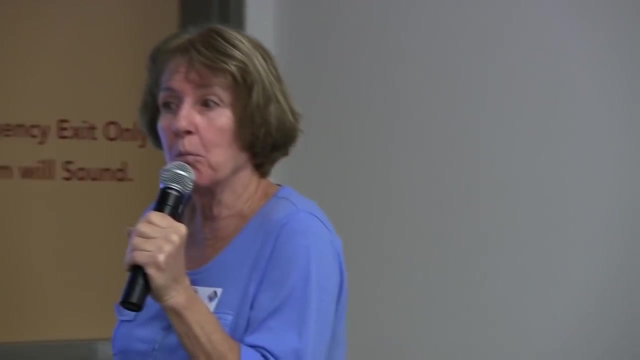 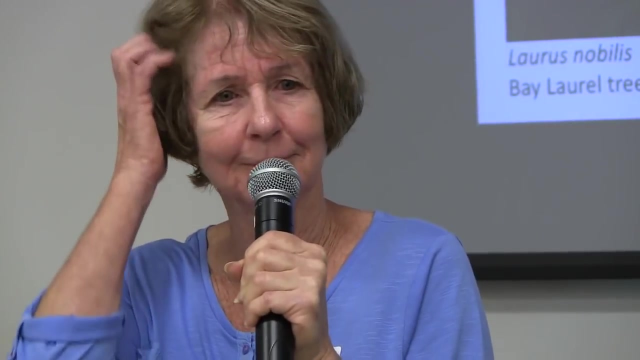 that I better smoke. I better soak it in a smoke solution before overnight, before I plant it, because that's what you do to proteas. If someone says, oh, I've got this euphorbia, you want to cut him, I go. hmm, latex sap can. 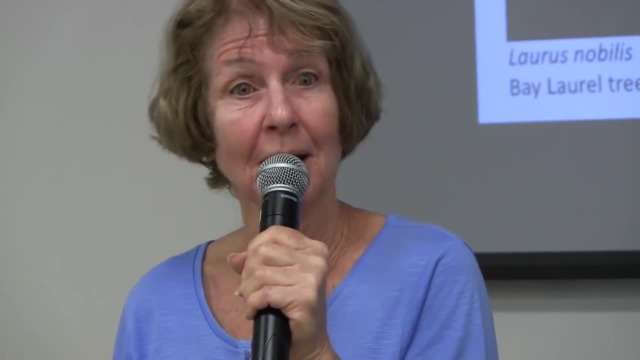 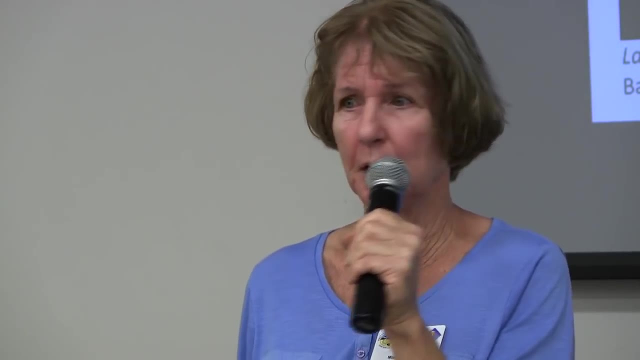 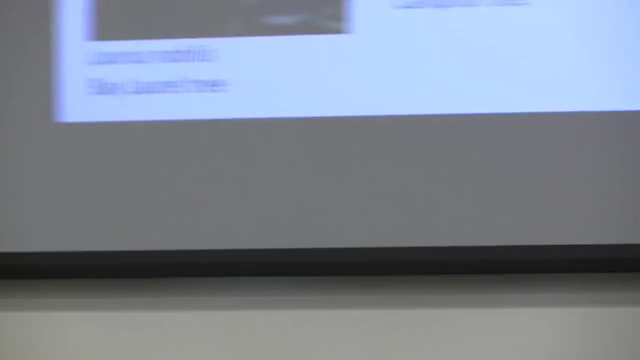 damage the eyes can damage the skin. hmm, maybe not, but you know that because it's a euphorbia. What else? The biggest family? anyone know what the biggest family is? Orchids. Oh well, see she, Laureen says orchid. 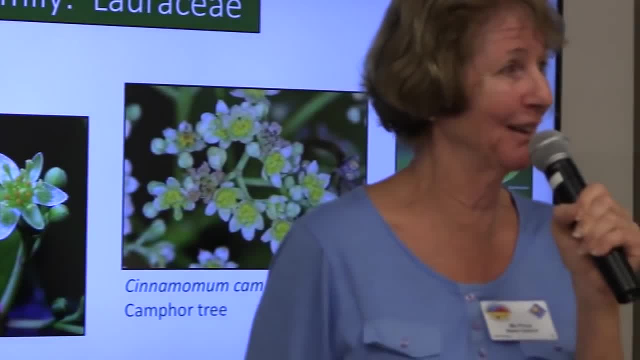 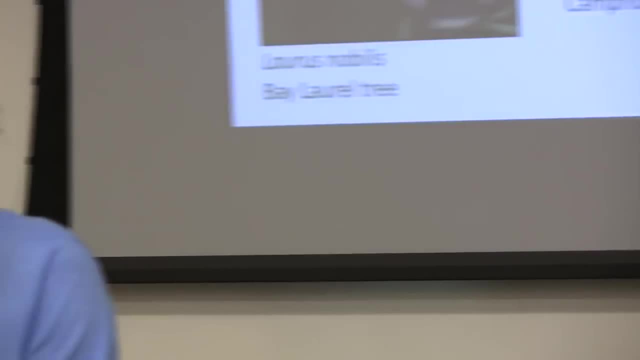 Others say asteraceae, Orchids, Orchid, Orchid, The asteraceae, the daisy family. Controversy over that. And then the third one is: the people say it's the Fabaceae family which is the legume. 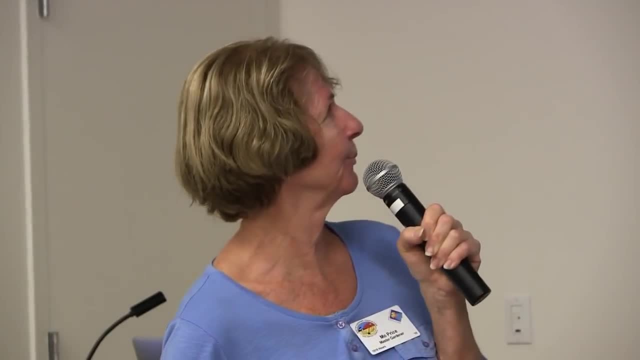 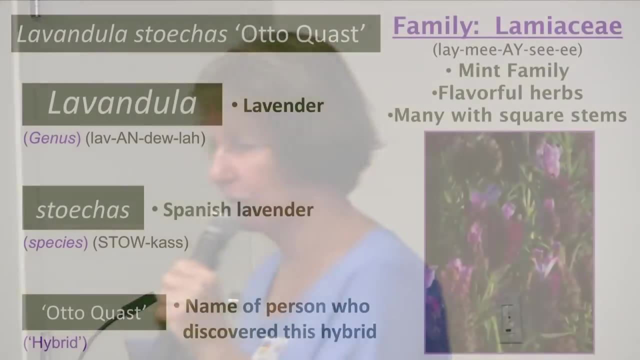 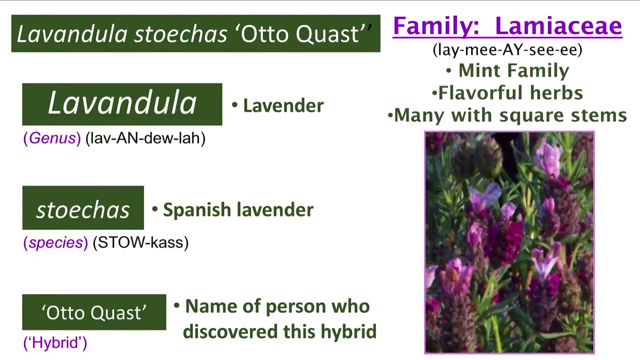 family. So knowing families helps. So let's look in detail at a plant family and genus and species. In this case we have the. what do we have? Lemaceae is Lamiaceae. as you can see on the top right, The pronunciation is there for you: Lamiaceae. 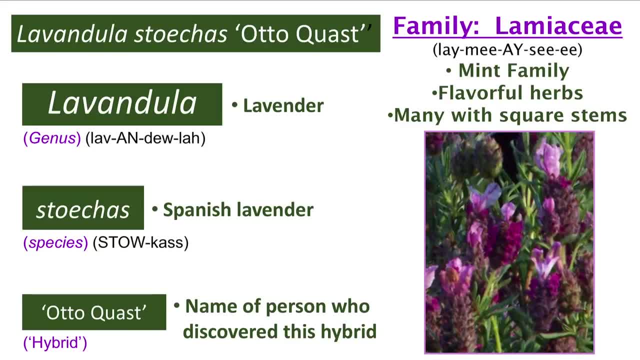 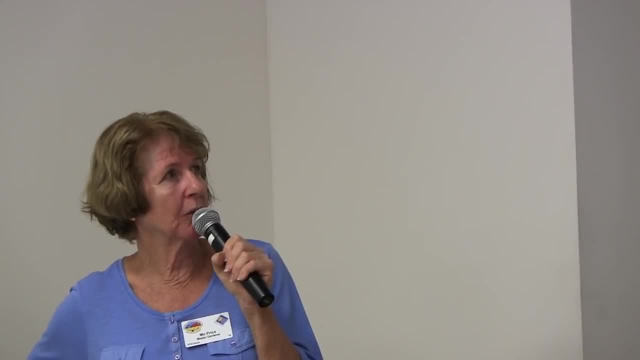 It also has an alternative pronunciation. you can say Lamiaceaei if you prefer, And the thing that's common about this family, the Lamiaceae family, is that the common name for the family is a mint family. It has many flavorful herbs and many with square stems. 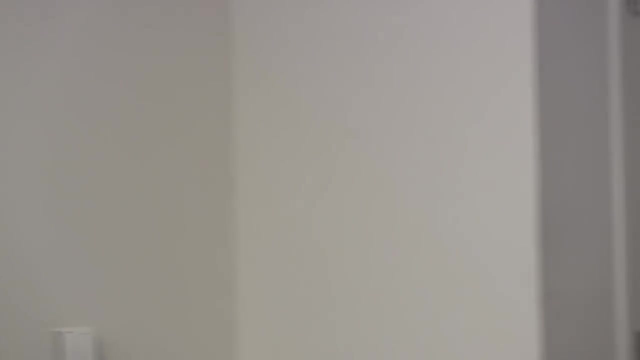 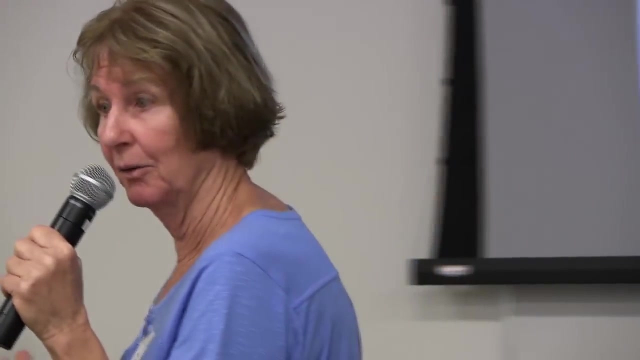 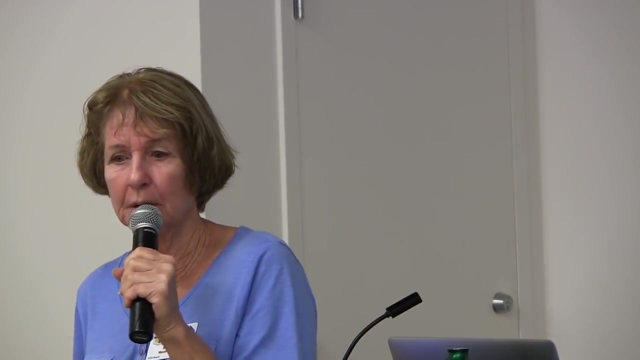 So you probably know some of the other plants in this family- basil, maybe, oregano, thyme, rosemary. They all have something in common, right? So that's what distinguishes the family. We are looking at a Lavender. The botanic name for Lavender is Lavandula, And this is 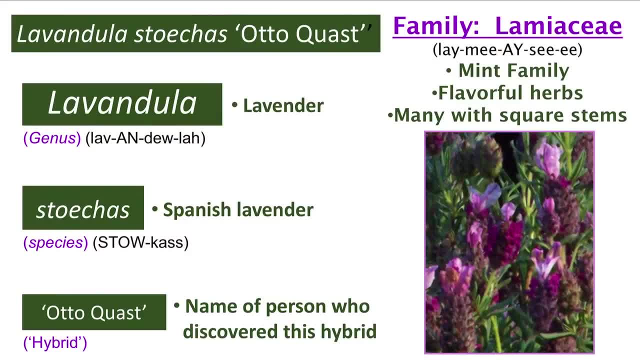 the genus, And, And so any plant in this lavender genius is a lower level, and the plants in the lavender family are all very similar in that they have similar flowers, fragrance and the leaves are pretty similar- Lavandula, If you take it down a layer further, and in this case this is Spanish lavender. 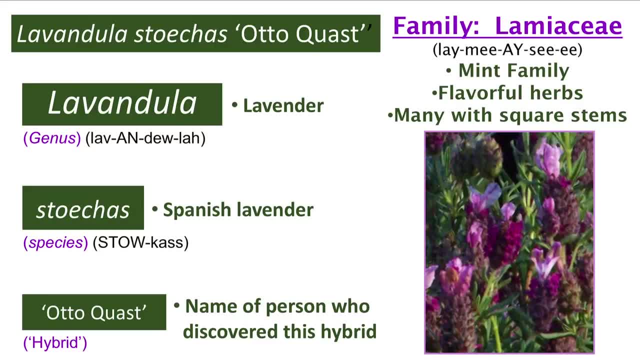 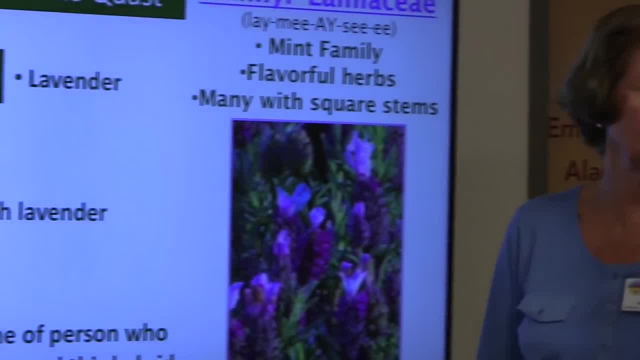 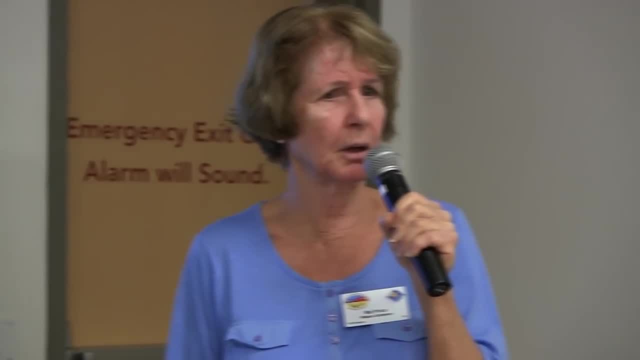 The slide that I showed you, a few slides back that had all the names on it. those are mostly adjectives that describe the plant and that's what the species does. It normally describes something about the plant And most of you probably have Sunset Garden books. 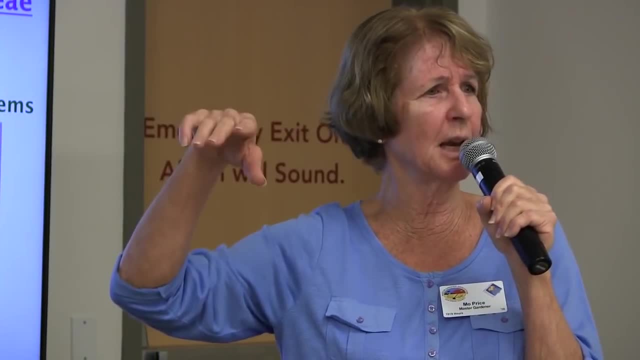 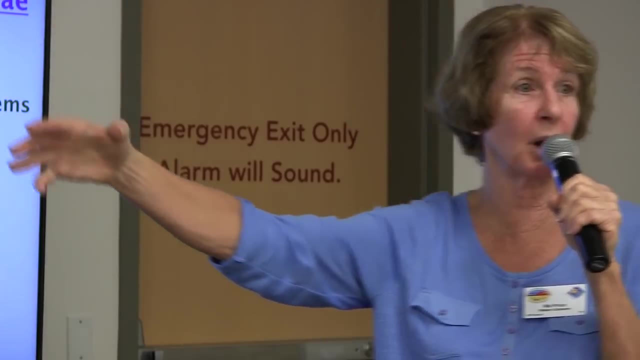 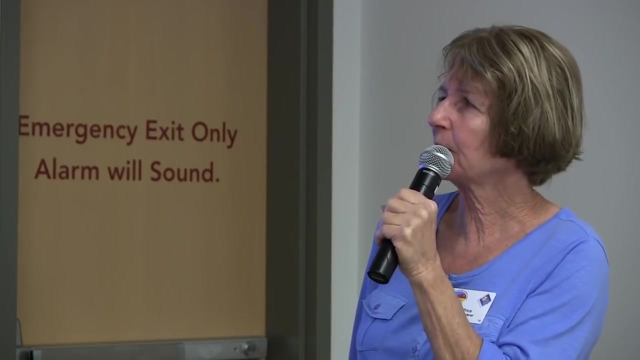 In the back of Sunset Garden there's a book called Sunset Garden. There are lists of botanic names by category, like categories that describe colors, categories that describe the shape of the flowers and other things. So that is an adjective, usually the species. 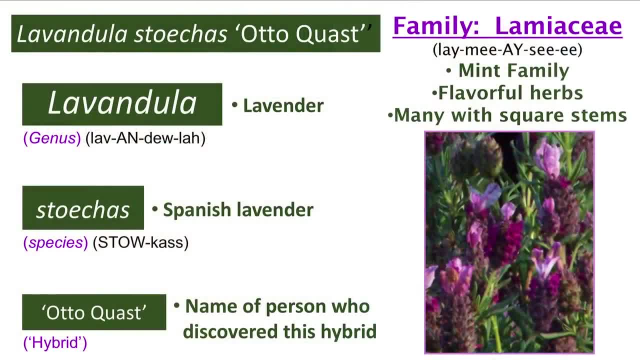 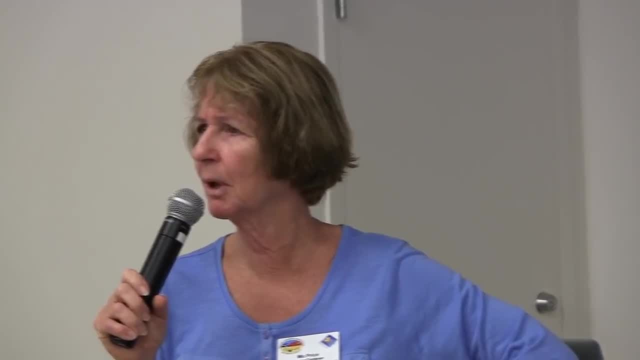 And then the last thing: if there is something there, it's the name of a person who discovered the plant or who breeded the plant. It could be something. It's usually some sort of hybrid. Oh, and I forgot to mention, on the genus, where the names come from, the genus names. 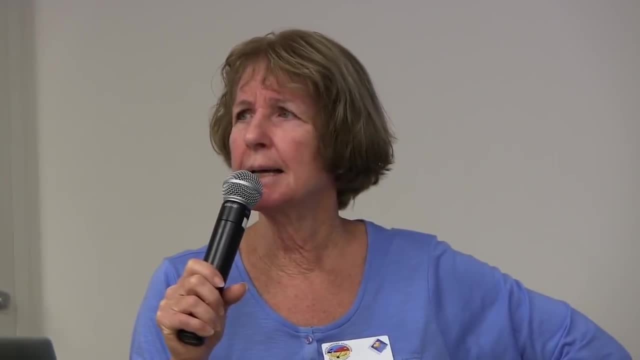 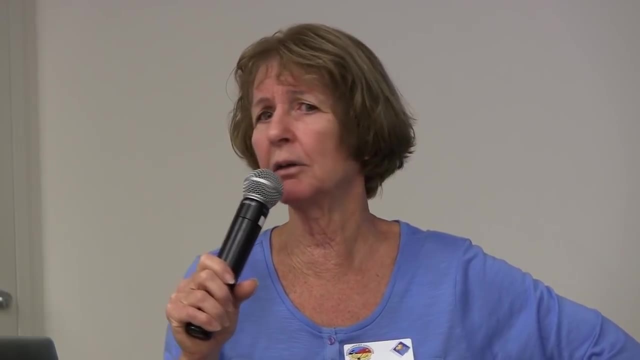 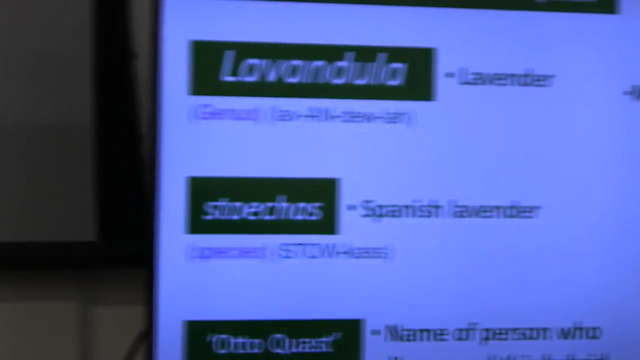 often the genus names are named after a person who did something remarkable, a botanist who did something remarkable, or maybe a botanist who discovered a plant. For example, the Banksia was discovered by Sir Joseph Banks. There's a genus called a Darwinia. 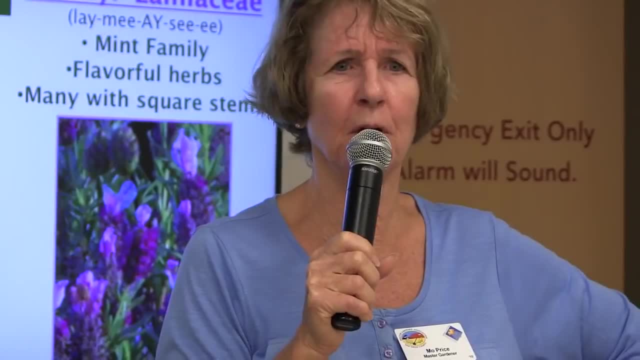 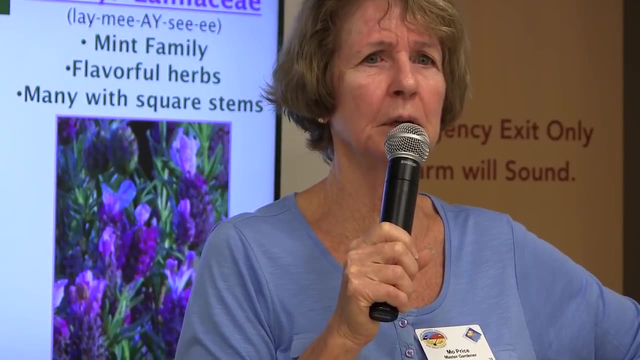 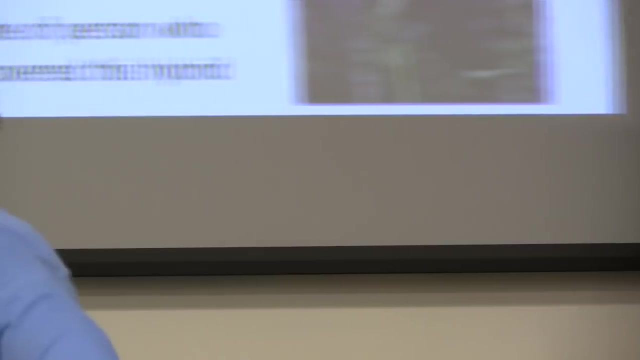 Darwinia. Any idea where that name came from? Anyone? Darwin, Darwin? What Darwin? Charles Darwin? This is a trick question. I'm telling you. Actually, the genus Darwinia was named after a man called Erasmus E-R-A-S-M-U-S. You don't have to write this down, It won't be on your final. Erasmus Darwin, who was the grandfather? He was the grandfather of Erasmus Charles Darwin. He was a physician, a philosopher and a poet, and he wrote. about evolution. He actually died seven years before Charles Darwin was born. Erasmus did, but he passed his information along and apparently Charles picked up on it. One other thing: the real reason why Darwinia is named after Erasmus Darwin is because Liz told you that Carl Linnaeus wrote his. 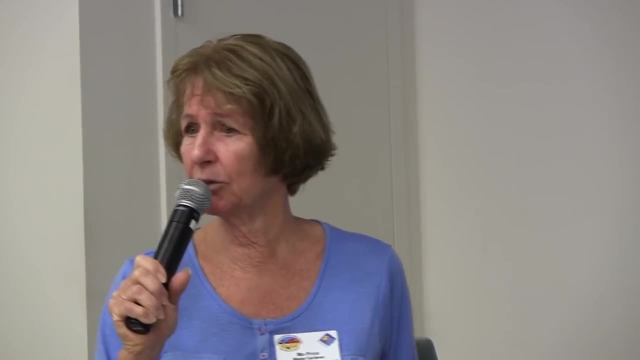 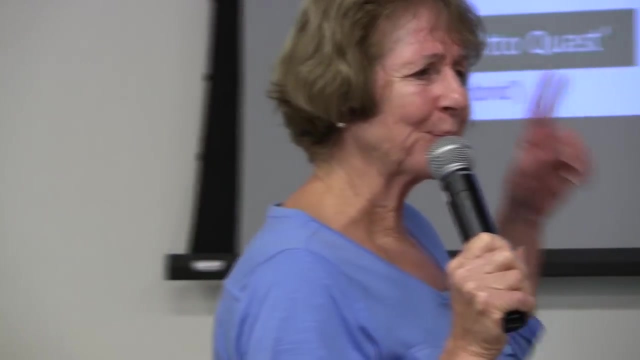 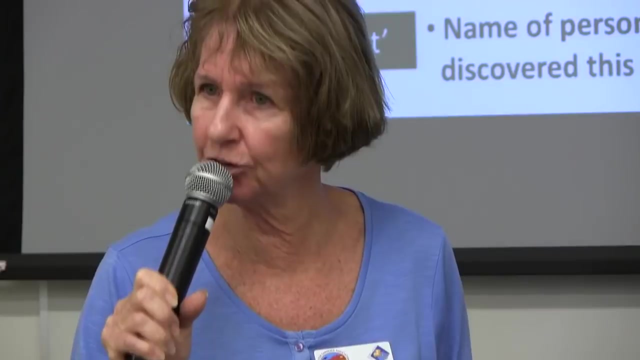 system, his binomial system in Swedish. Well, who can read Swedish? huh? So Erasmus Darwin translated Carl Linnaeus' works from Swedish to English, and that's why he got the genus named after him. So there are reasons why this happens, Isn't that? isn't that an interesting story? Is there a? 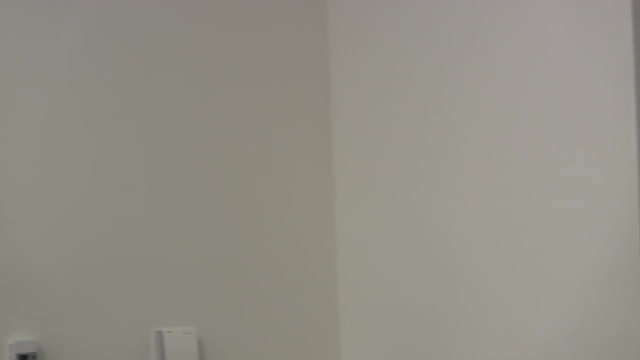 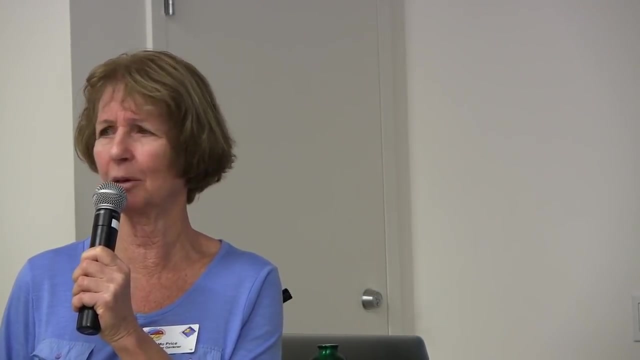 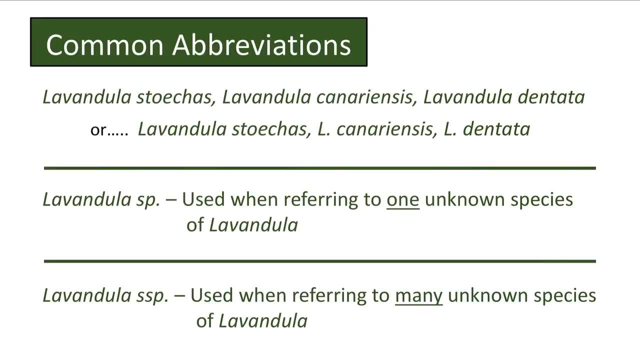 Darwin, Erasmus, Darwin, Erasmus, Darwin, Erasmus. Now, it's a lot of work to write lavandula, and if you're writing about plants, maybe you know you're doing a presentation or you're writing a paragraph. it's a lot of work to write. 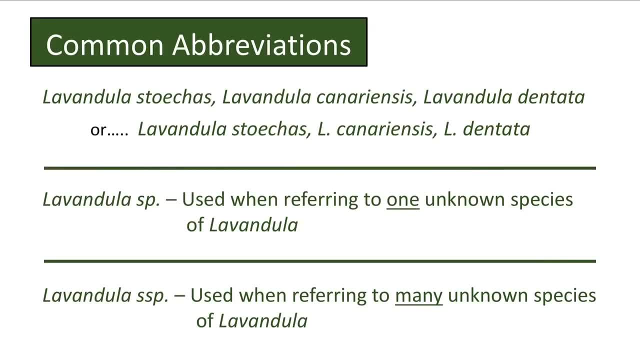 lavandula stoches, lavandula canariensis, lavandula dentata. So we make it simple, Or someone made it simple. Once you use lavandula stoches, you can. after that you need to keep it, like in a paragraph or in the same page. you can. 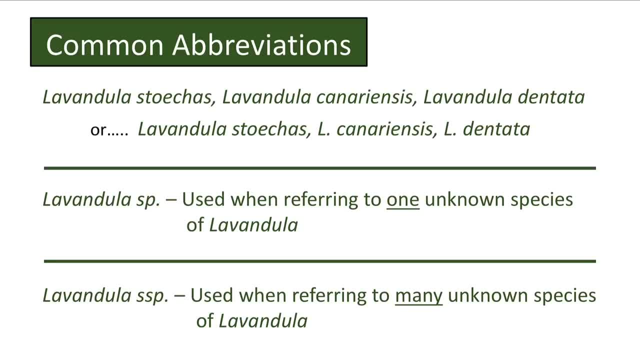 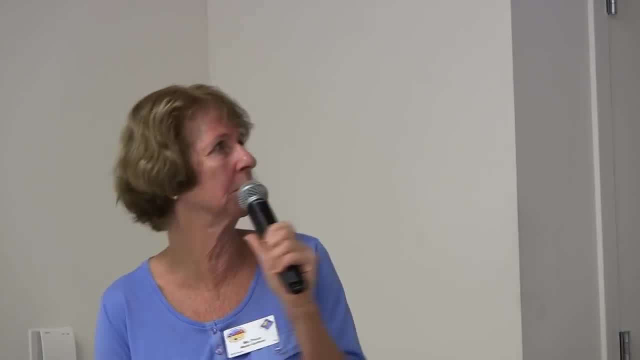 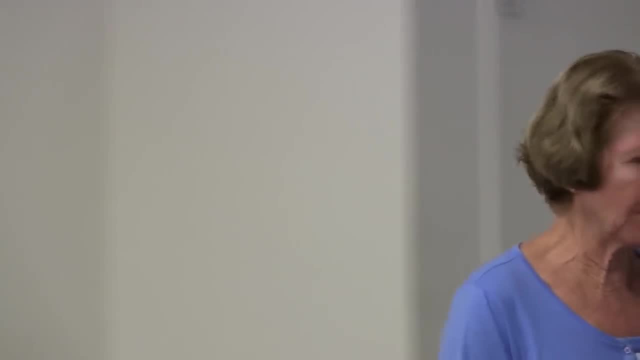 just have a capital L, as we have here, period, and then canary ensis for capital L period, then Tata, you don't have to write the whole darn level whatever. it is not a doula out every time another comment, abbreviate or another abbreviation is. if I'm doing the presentation and I took a picture of a. 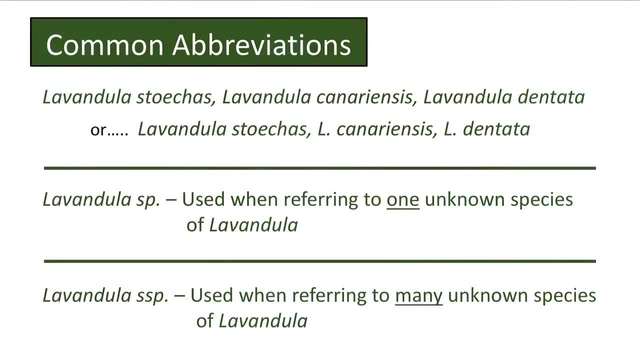 lavender. I should really, and I don't know the name of it. I would write lavender love, SP period, and that means, is that some particular species of lavender, but I don't know what the heck it is? or if I have many plural I would key in, I would write SSP or several. I'm referring to several unknown species. 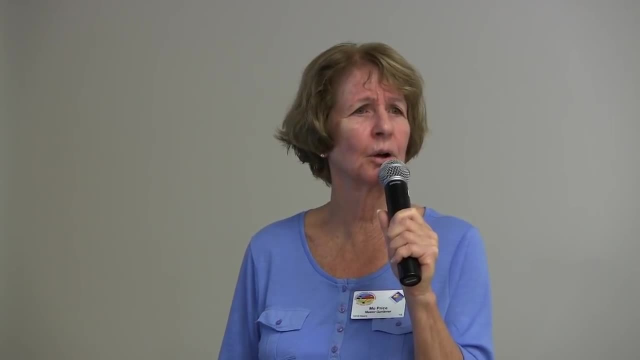 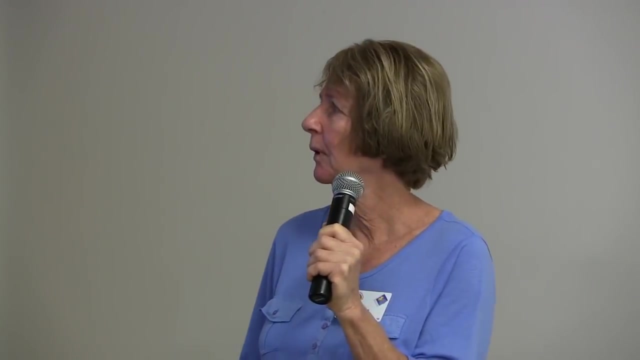 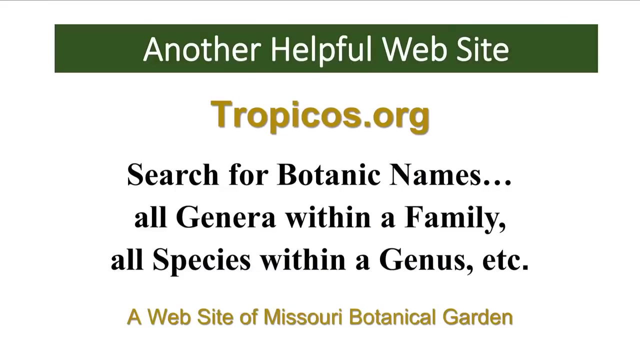 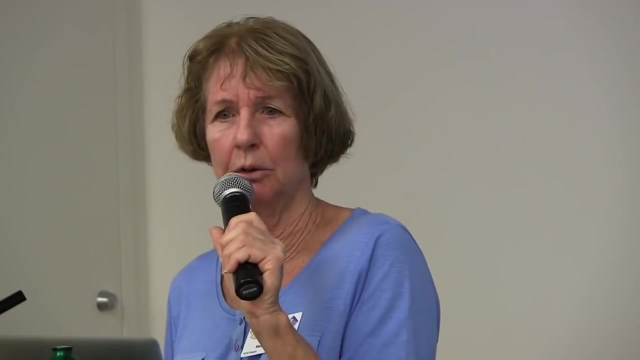 simple enough, Liz, subspecies. thank you. there's another helpful website here and this is called tropicals. tropicals- it's the website of the universe- was the Missouri Botanical Gardens. the website has a lot of useful information on it and you can find out interesting things like which plants are in a family, which 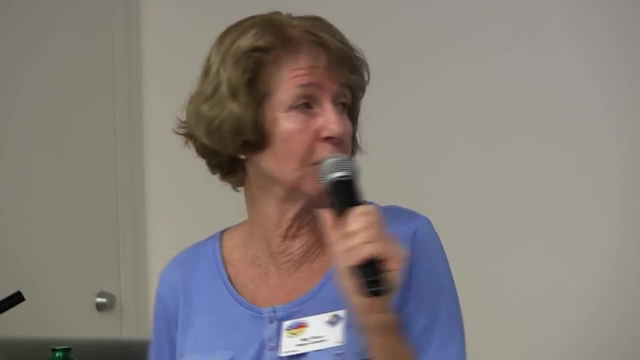 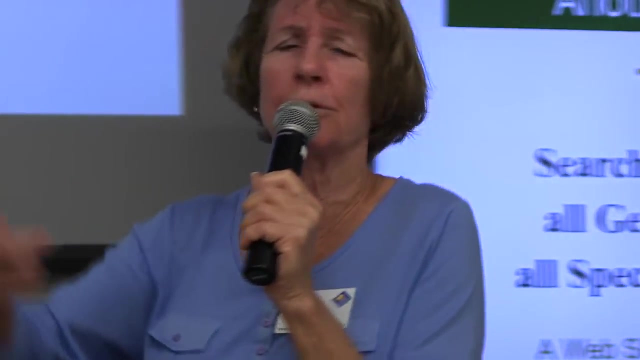 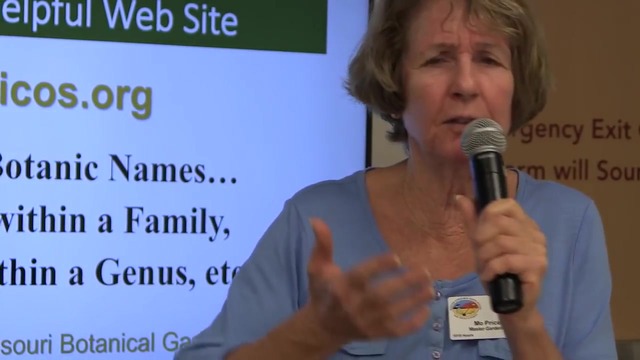 G nus are. the species are very helpful and I you need to find information. I'll use that. one other thing: yeah, I highly recommend you learn the boat. oh, one other thing: I highly recommend you learn the botanic names, but- and I I've learned them, but I don't get carried away if I see a field with beautiful orange. 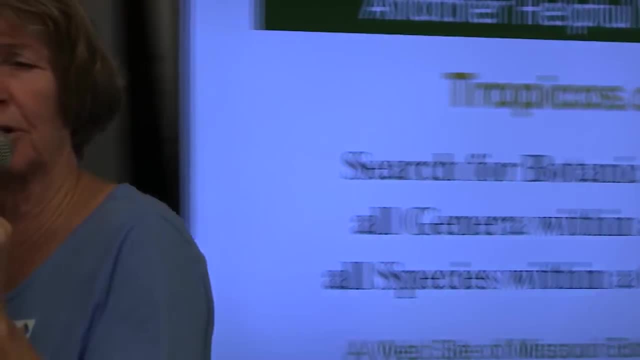 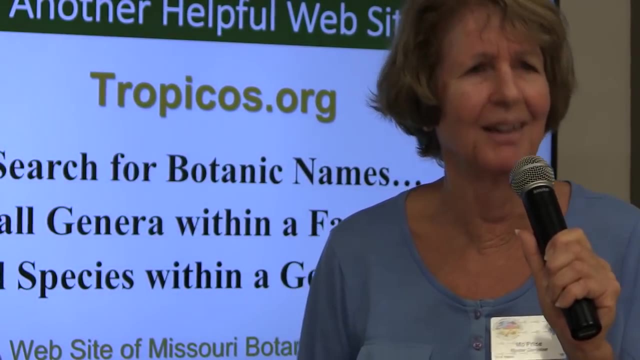 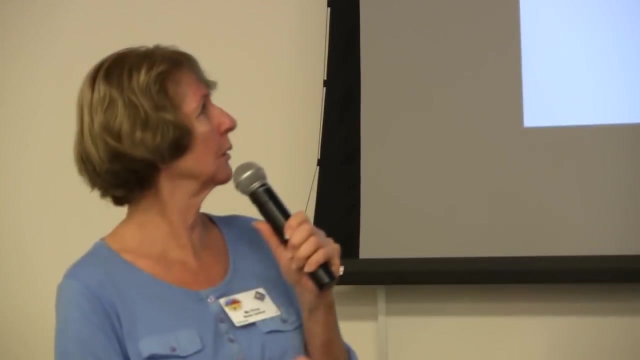 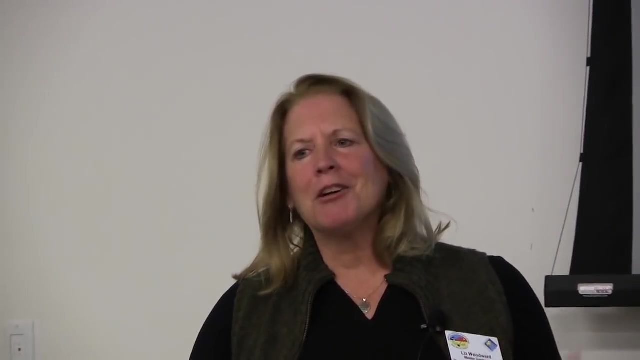 flowers. I would say, oh, look at those California poppies. I wouldn't say, oh, look at those beautiful, as you'll see, as Californica's there are some and I think, I think that is the end and, as most said, it's important that you know, you learn those botanic names or you know, especially if 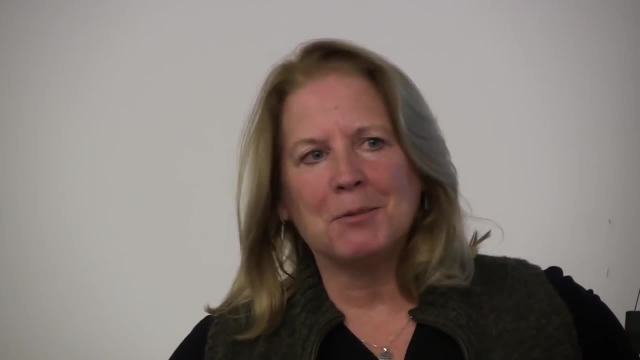 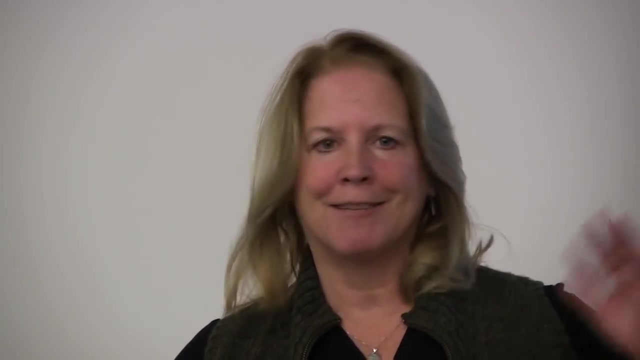 you're into a particular field, you know when all those vegetables out in the garden have botanic names and you would almost never refer to a vegetable by. you know a tomato by I can't lyceum or whatever it is. you know it just in some. 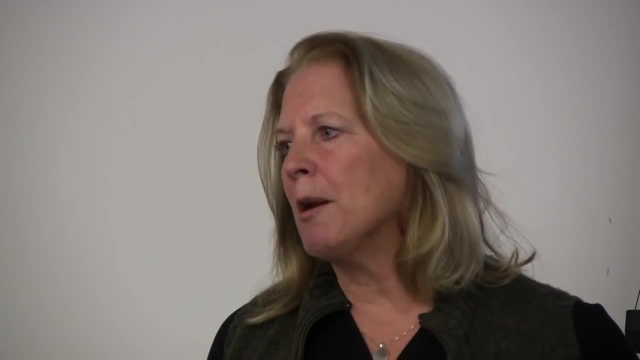 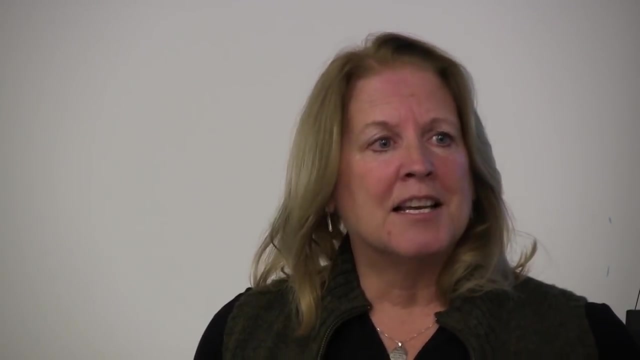 areas. it's just not done. but you know, especially with your ornamentals, and if you know for those, you know anytime you're working in the landscape business or you know- and again you do use that if somebody is sending you something to the hotline and you're identifying it because, as Mo pointed out, they have they. 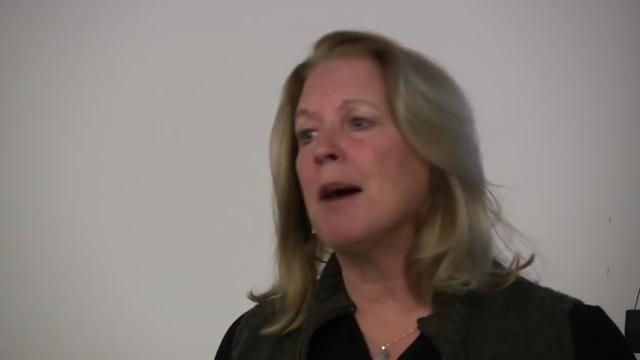 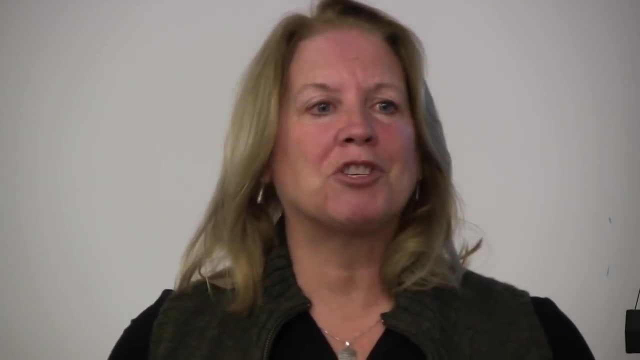 have a lot of. there's a lot of common names, so, and a lot of those common names are regional. so if you come from a particular area, you know I always think of, like the snow and summer plant which is like it's, it refers there's a there's. 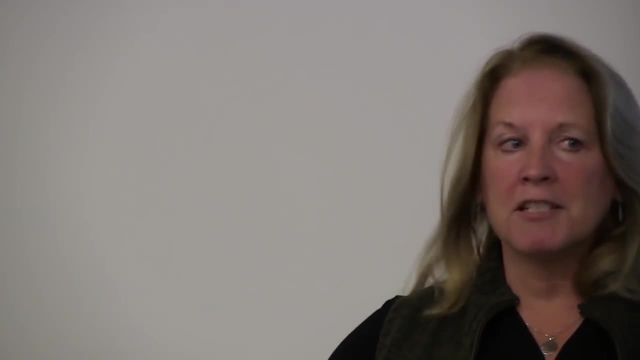 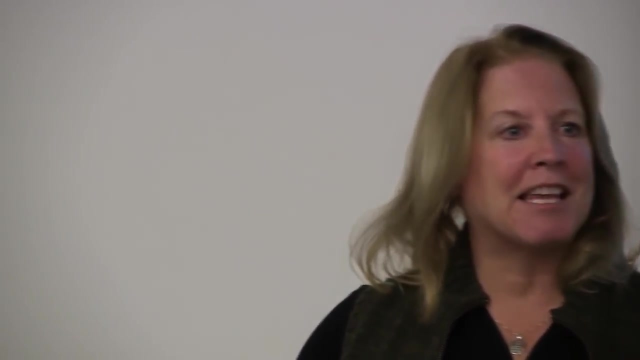 a plant that's a ground cover, and it's a plant that's a ground cover, and it's a ground cover that's called snow and summer. and then there's a big, huge tree. that's also called snow and summer. so if somebody comes in specking out that they 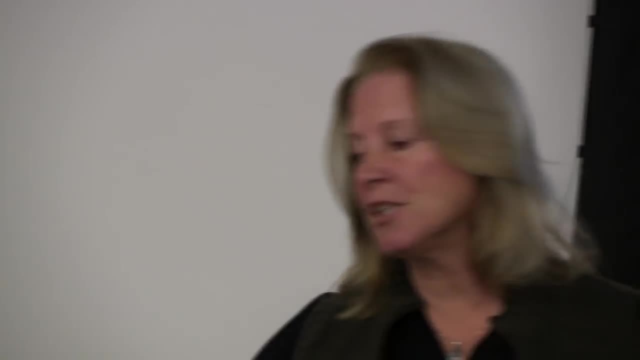 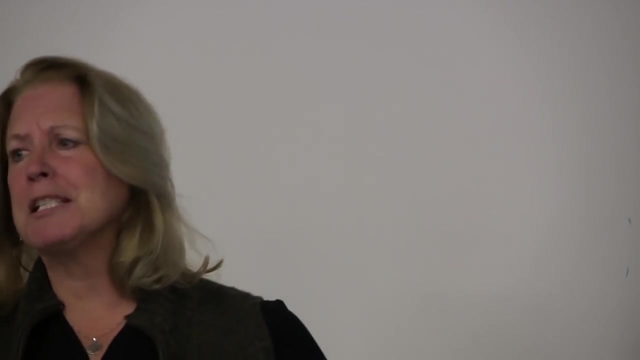 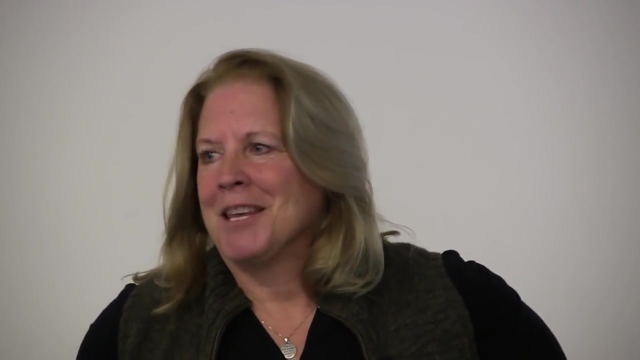 need five: snow and summer. you better figure out what it is that they need. so that's why it is it is important that we use those or get familiar with it. but you're always speaking to your audience and that's one thing I think. sometimes people are turned off sometimes when we talk in the Latin at them and you know. 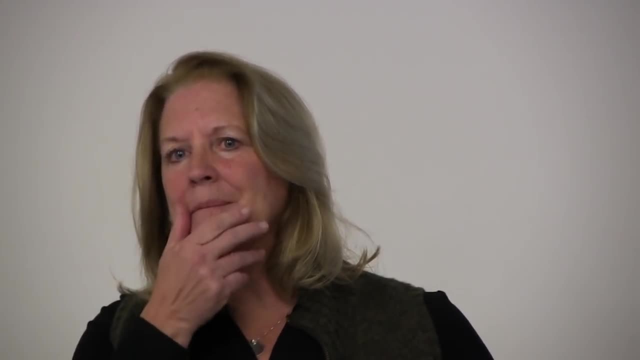 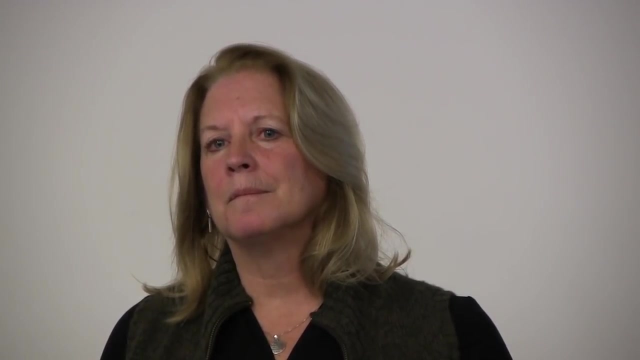 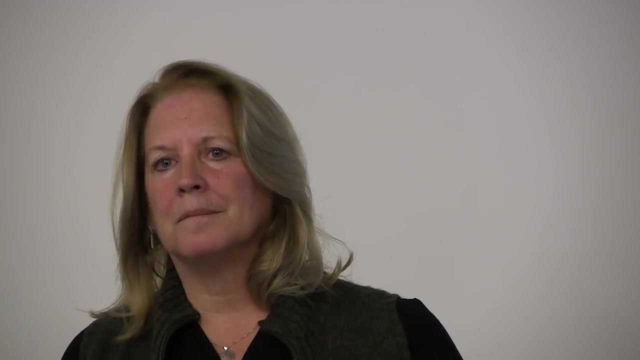 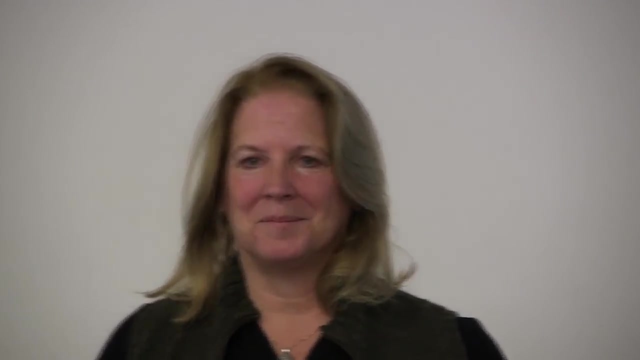 so just you know, depending on who you're speaking with. yes, we were the first got yard and our homeowners association put a name of a drop taller fence above the grass in our front yard and we used to put the botanic names on every fence because people were knocking on our front door constantly, and so now it's out there and they take pictures of the ground. 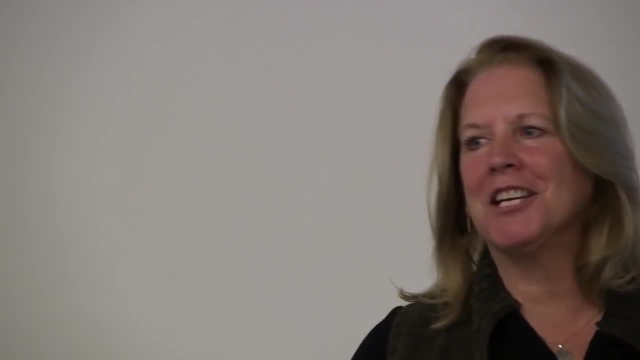 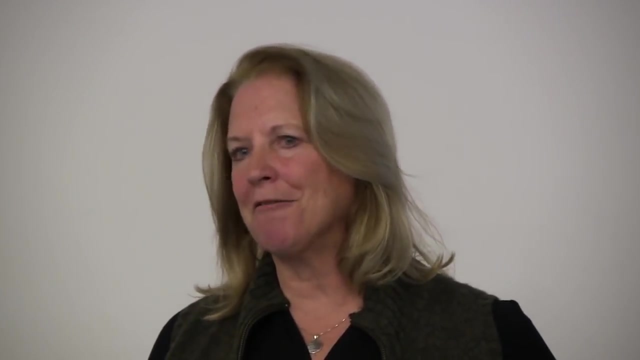 okay, and she's commenting that in our home owners association that they read it a lot. right, that's myấn landscape and they people. because again, people were asking in them them what it was, they ended up labeling it in their front yard, which is a great way to to do. 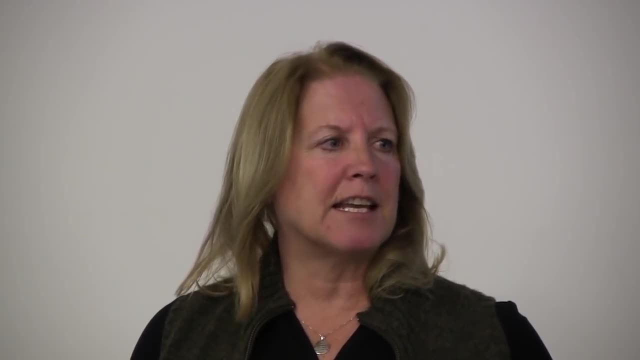 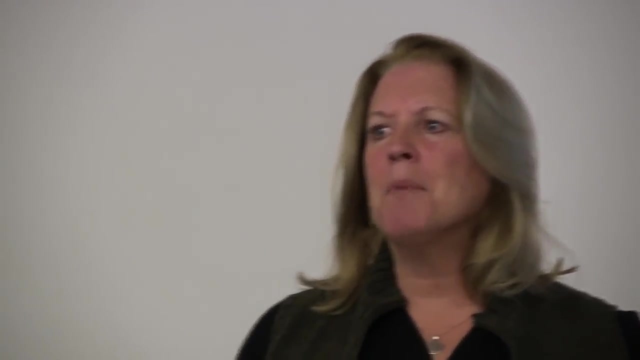 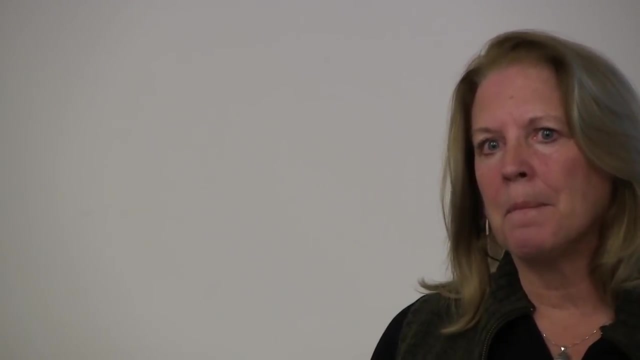 it and you, when you go on garden tours, you'll often see like, especially things that are, you know, done by like, the San Diego Horticultural Society, and if, when things are labeled, most times you will see on garden terms that things are labeled usually with both the botanic name and the common name on there. so 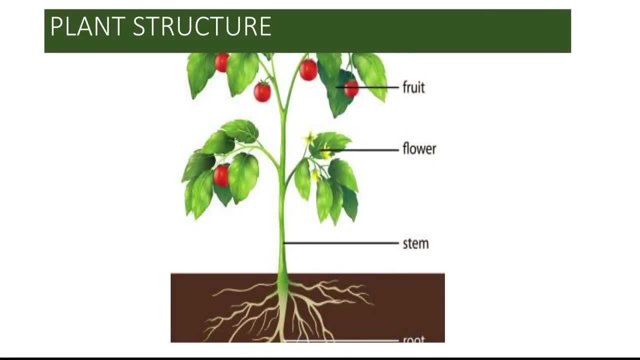 we're going to be moving into plant structure and basically there are two parts of a plant. there's the vegetative structure and the the, the sexual reproductive parts of the, of the plant. so in the sexual reproductive parts are like your, your bud, your flower bud, your flower and your seeds. the vegetative 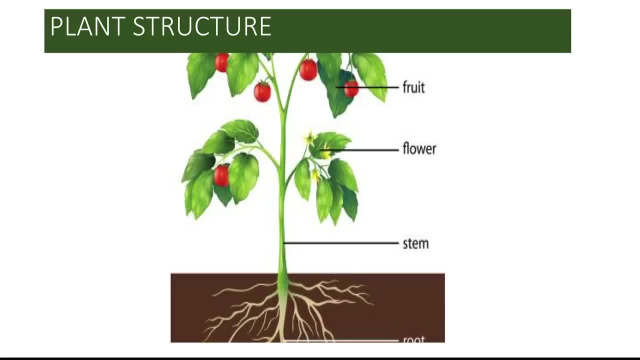 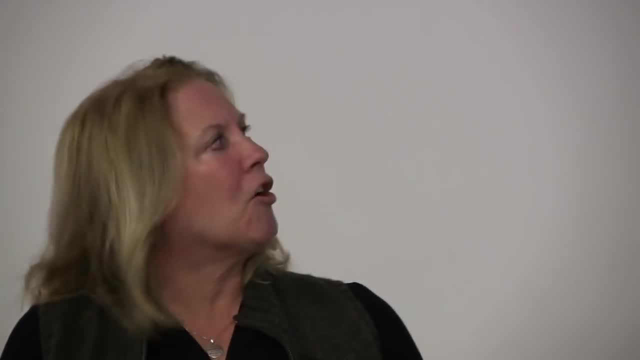 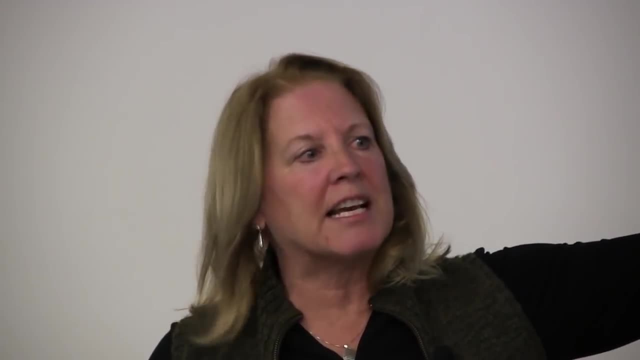 parts are your roots, the stem and your leaves, the, and there are. there are parts like you could say. there's an argument you could say that, like when we do, when we do certain propagation using cuttings, we actually are using some of the vegetative parts for reproduction, like 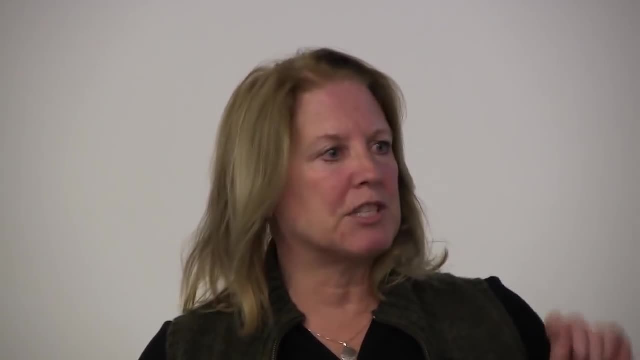 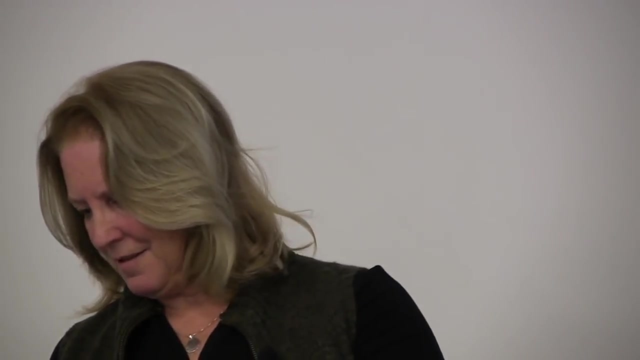 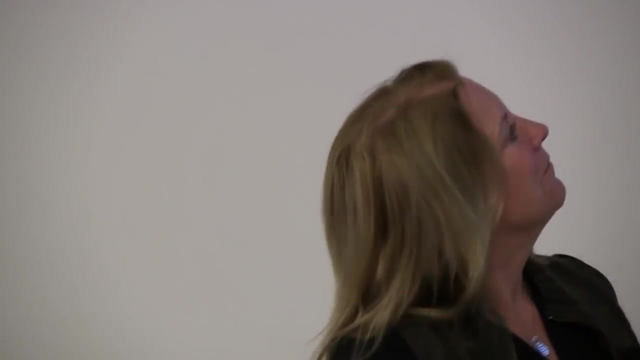 if you've ever tried to especially. we see this a lot of times with succulents. we're just sticking a leaf or a part of a plant and propagating, and I think you're going to get into that. no, do you have the? this is probably a part of a plant that most of you have. 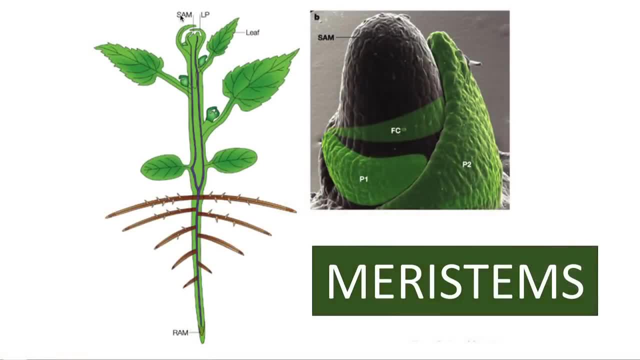 never heard about the which one most important parts of vegetative parts of the plant is the meristem. and it's really not. it's so much a part of the plant as it is kind of tissue in certain zones. meristems occur at many of the 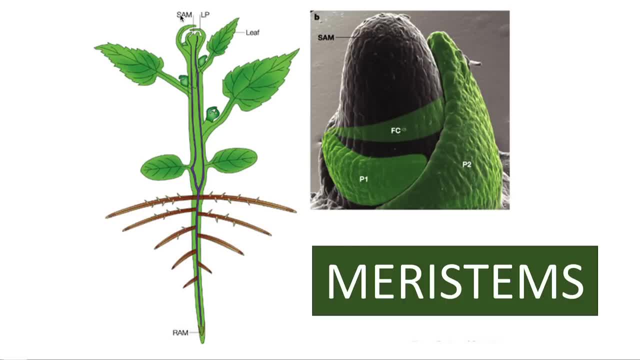 vegetative parts of the plant and they're responsible for that's. it's a thin layer of tissue that occurs both at the root level and usually at the at the growing tips of a plant and at the at the bud apexes that give it that it is. it is where the growth will occur. it's largely composed of water. the meristemic areas get most of the activity from the plants, like most of the energy and food that's going to that plant, especially as that plant is young and growing. are going to the are going to these regions because this is where the growth 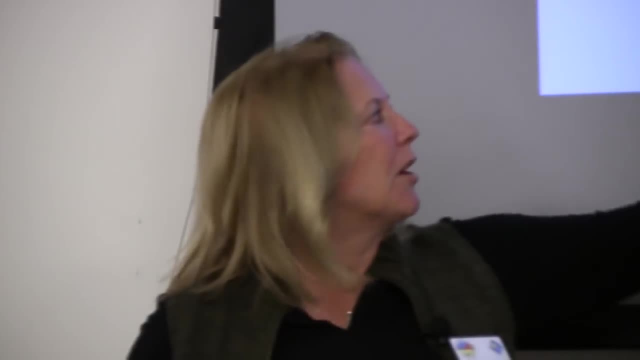 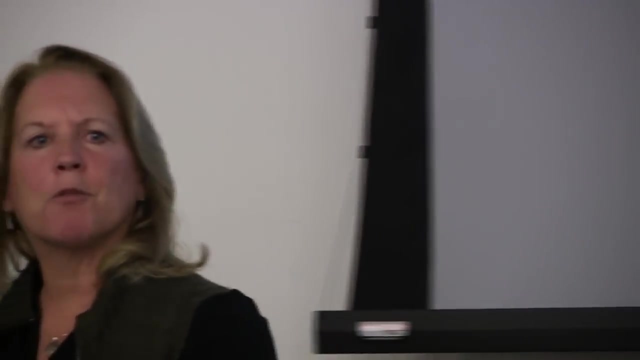 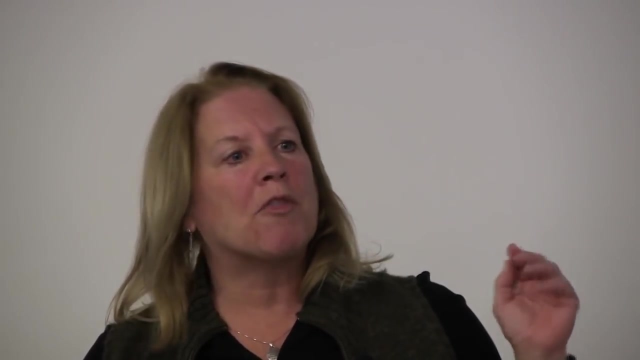 will occur, the again typically in the root area. we call it a- I think, a radical something- meristem. it's the root, is giving the plant energy for the root to to embed itself in the ground and to grow quickly to get that plant started. and same thing at the tips and where this becomes important to you as 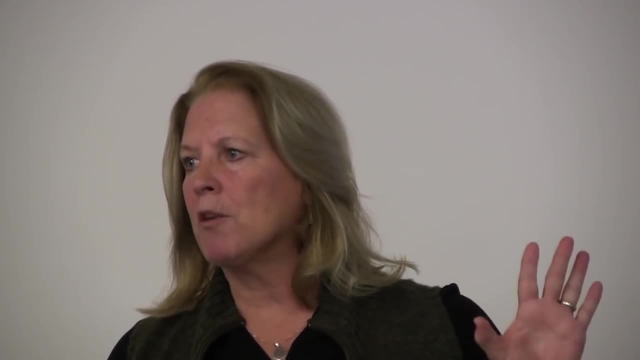 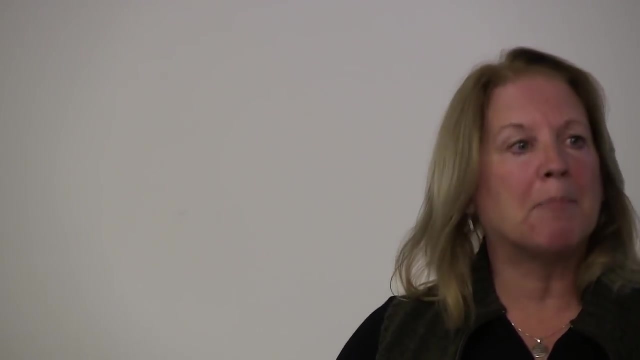 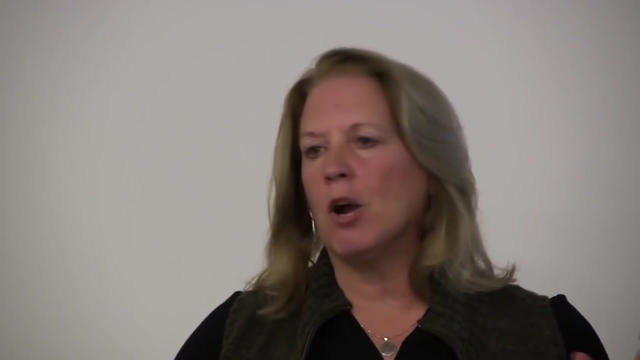 gardeners and advising people is understanding kind of where those meristemic tissues or cells are in a plant, help you as you get into into pruning a plant plant for optimal growth. you understand where the growth is occurring, when it's occurring, some of its occurring by, you know, at the age of the plant obviously. this is growing really quickly when a plant is really young and growing at a point- sometimes with a mature plant, you notice how your orange tree when you plant it takes a certain number of years to get to maturity. a lot of the meristems in that orange tree are looking to again develop that root in. 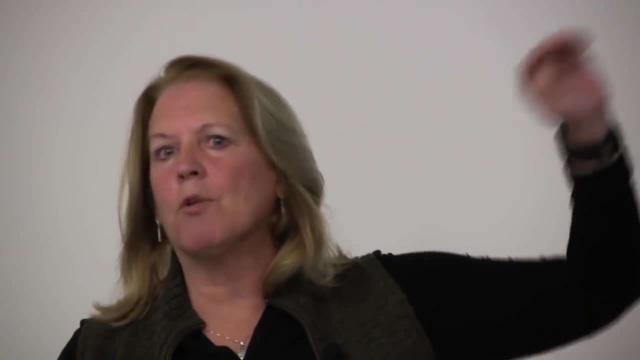 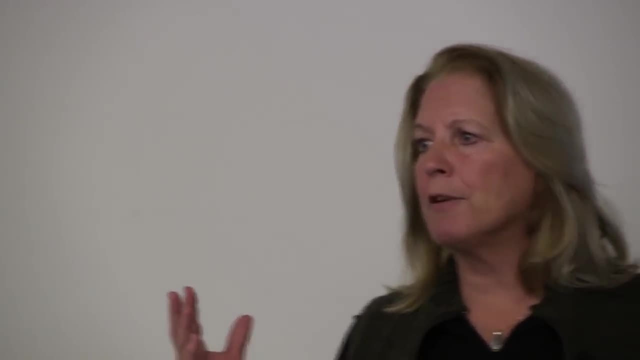 the ground develop. you know, get those leaves going, get those the meristems going, put wood on that tree, getting it ready. and sometimes it takes a while. you notice, when we plant a lot of our fruiting plants, it takes a while for it to actually produce its flowers because the energy for that plant is.